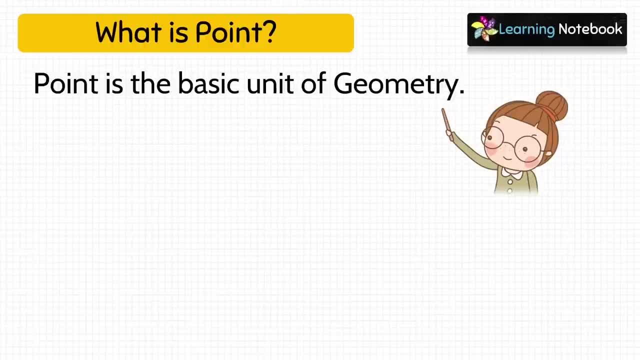 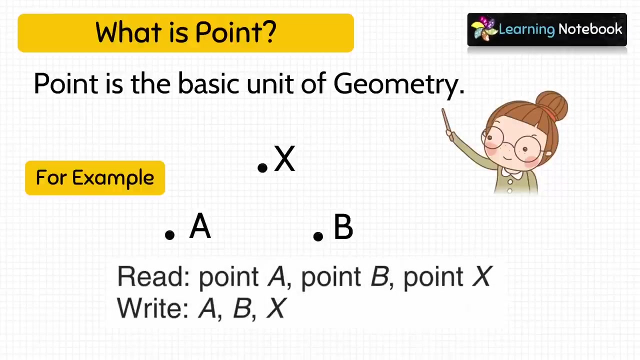 That means a point has no length, breadth or height. A point is represented by a dot And it is named with a capital letter. For example, this is Point A, Point B and Point X. So how do we read this? 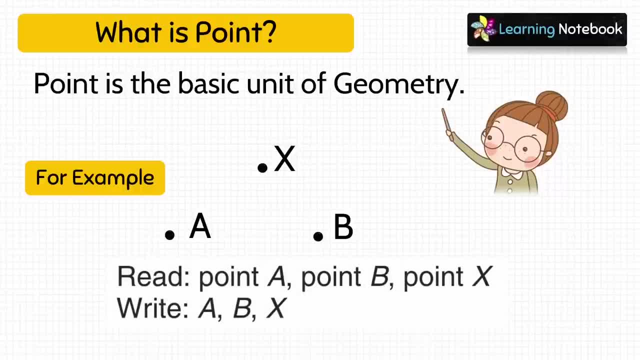 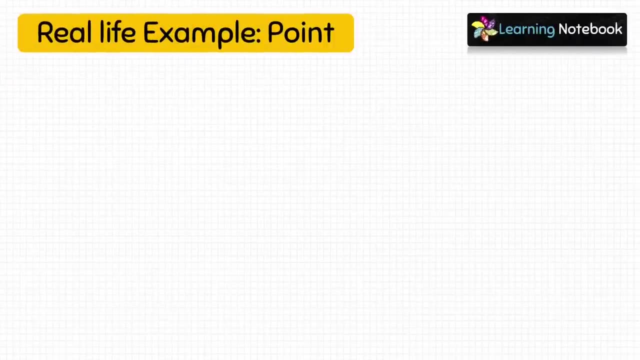 As I just told you, we will read them as Point A, Point B and Point X. And how do we write these Points? We will write them as A, B and X. Let me tell you a real-life example of a Point. 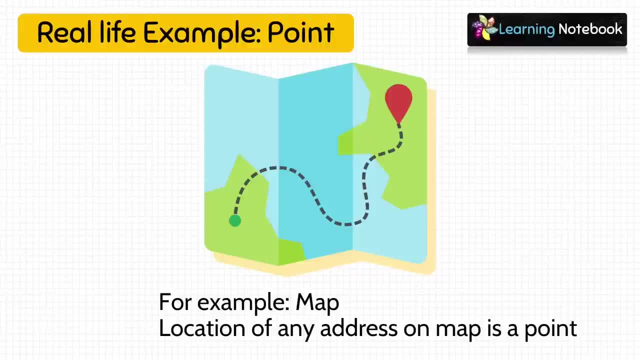 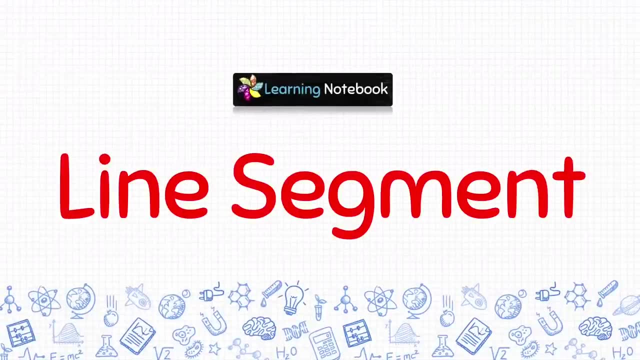 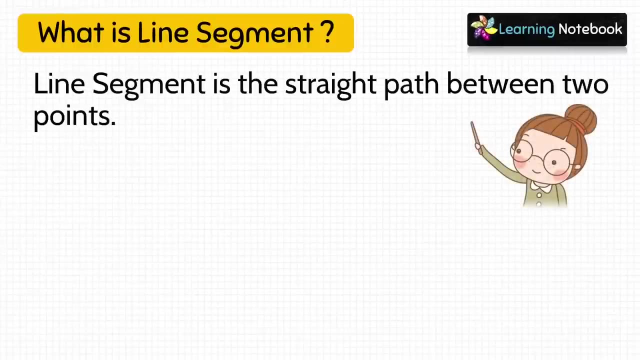 For example, Location of any address on map is a Point, Next is Line Segment, Next is Line Segment. A line segment is a straight path between two points. It is the shortest distance between two points. For example, there are two points DE. 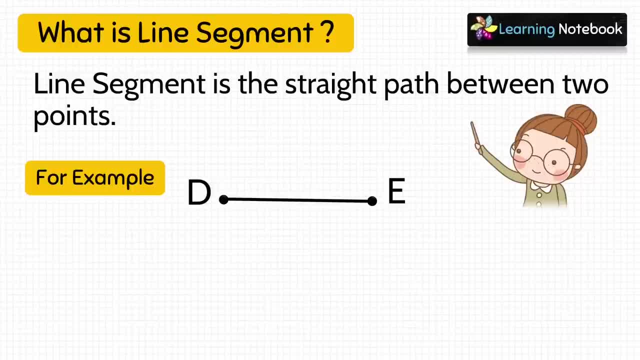 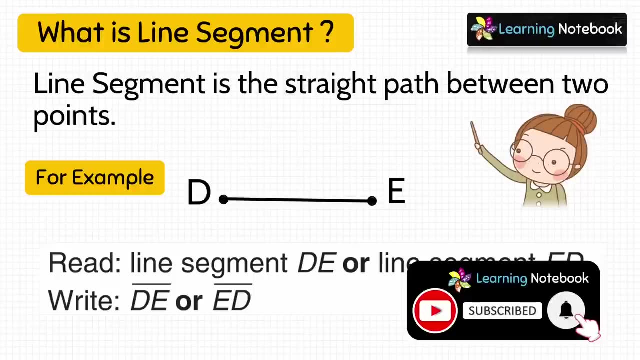 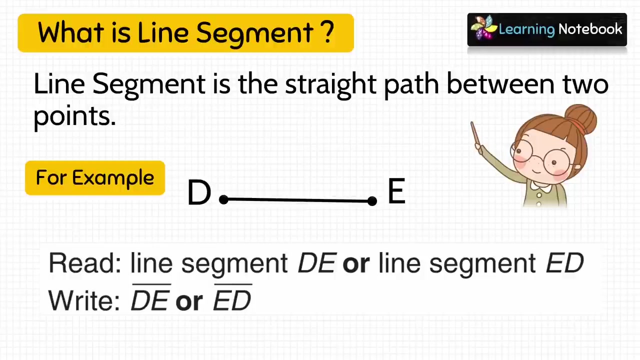 So line segment is the straight path between these two points. Now let me show you how to read and write line segment. We will read it as line segment DE or line segment ED. both the ways are fine. Similarly, we can either write it as DE or ED, with a small line segment on it. 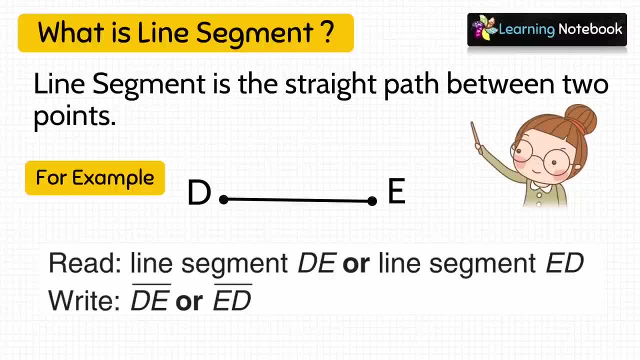 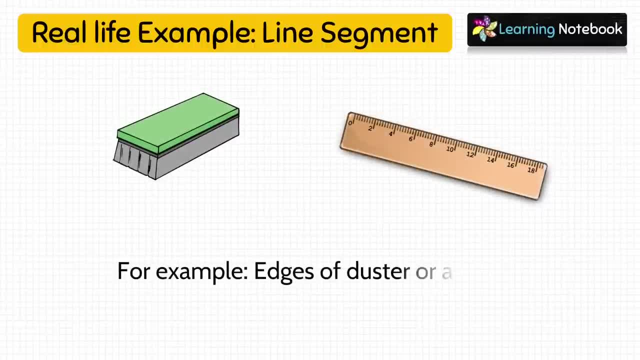 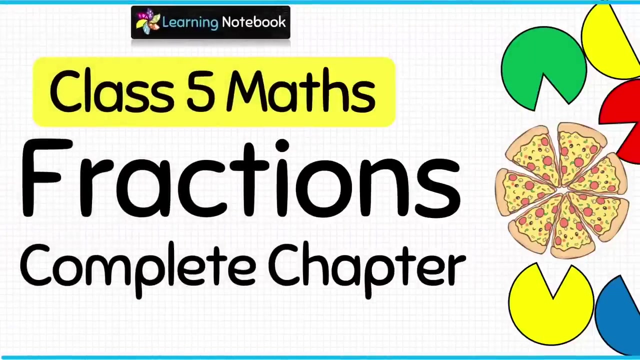 Also, students do remember that a line segment has a definite length. Now let's see some real-life examples of line segment: Edges of duster or edges of a ruler. they are line segment because they have a definite length. Students, we have a separate video on complete chapter of fractions for class 5.. 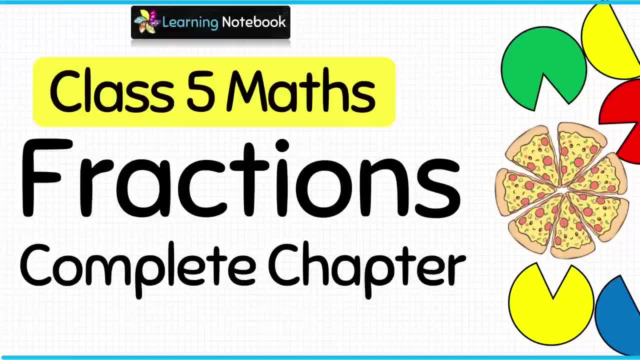 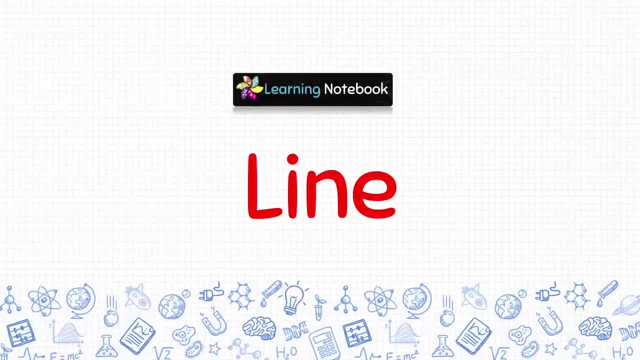 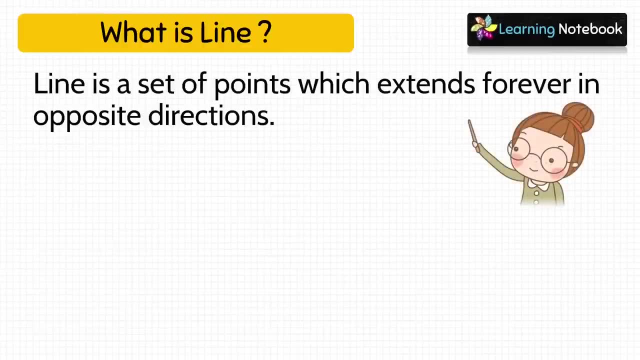 I would recommend you to watch this comprehensive video. The link to this video is below in the description box. Next is line. A line is a set of points which extends forever in opposite directions. For example, this is a line. The arrow on its both sides represent that a line goes in different directions. 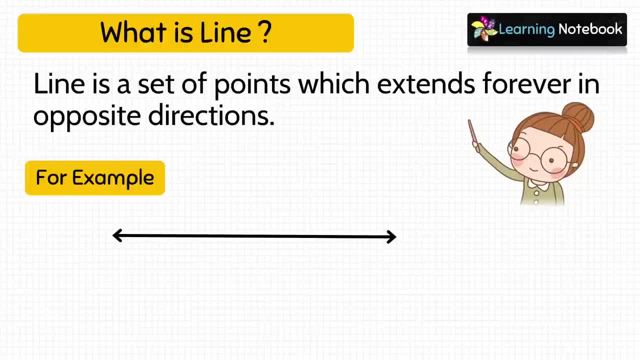 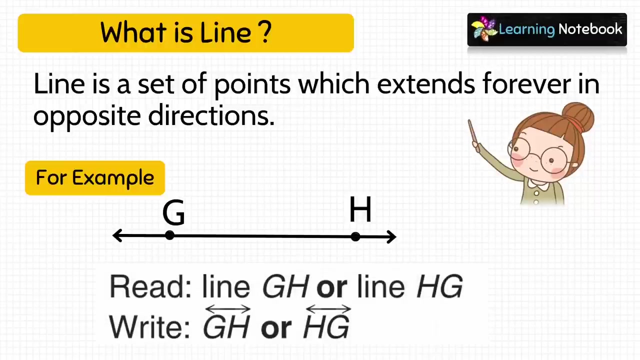 So, students, it means a line has no fixed length. Now let me tell you how to read and write a line. For this we need to take two points. Let's take G and H, So we read a line as line GH or line GH. 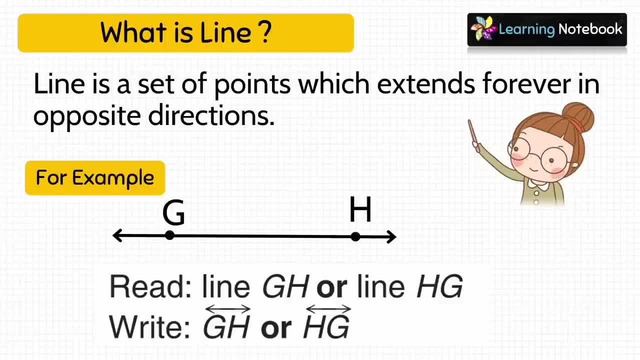 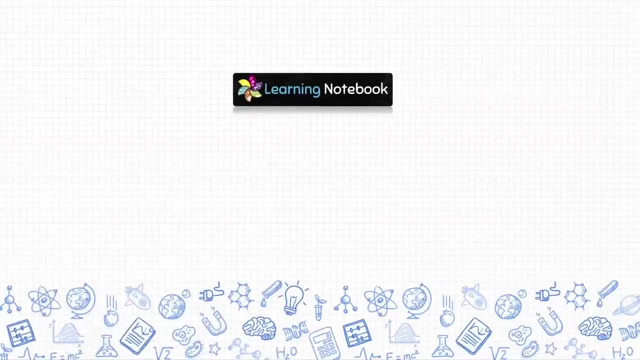 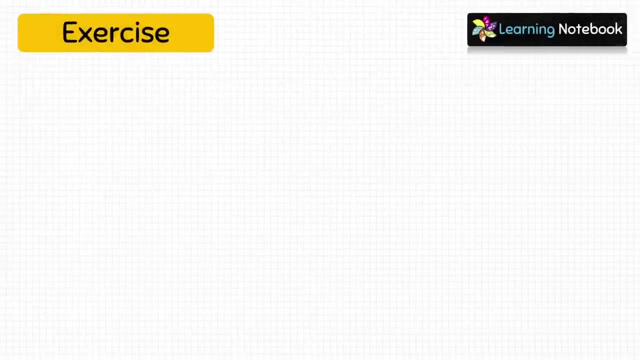 So we read a line as line GH or line GH. Both the ways are fine. Similarly, we can write it as GH or HD, with a small line drawn on it. Now, students, to revise these concepts, let's do an exercise Here. we need to identify line and line segments. 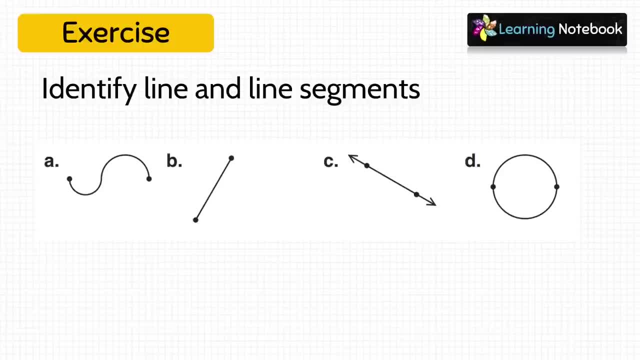 Here we need to identify line and line segments. Here we need to identify line and line segments. First, take a look at figure A. A is not a straight path, So it is neither a line segment nor a line. Now take a look at figure B. 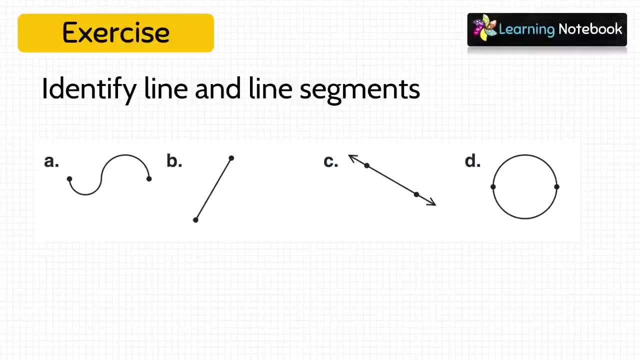 It has two endpoints and has a definite length, So it means it is a line segment. Next, look at the figure C. It has two arrows, So it means it is never ending. Therefore it is a line. And the last figure- Again, the last figure- is not a straight path. 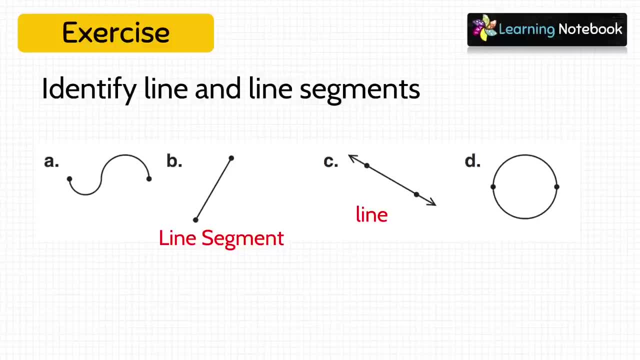 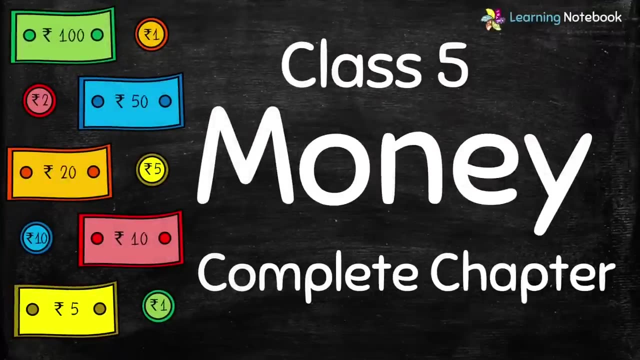 So it is neither a line segment nor a line. So, students, now I hope you have understood the difference between line and line segments. the difference between line and line segments. Students, if you want to understand each and everything about money, then do watch our separate video. 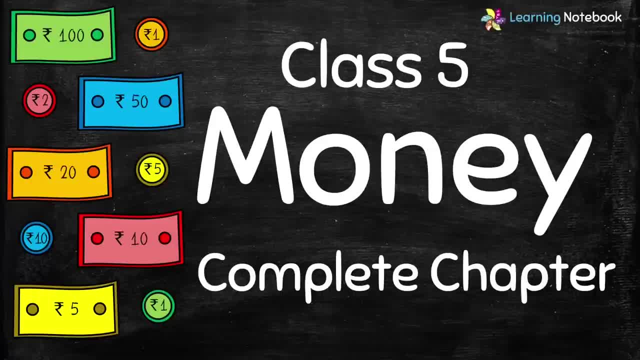 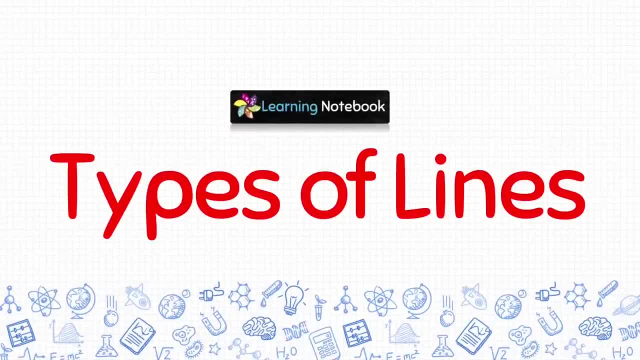 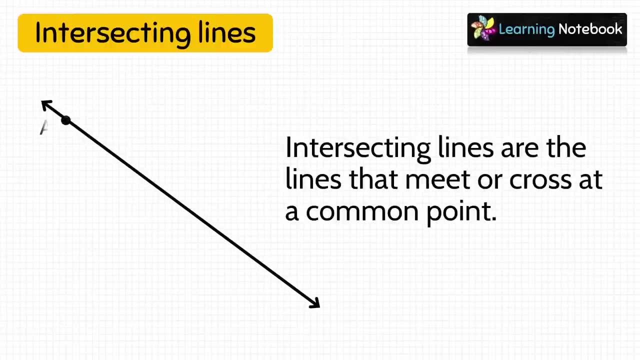 then do watch our separate video. The link to this video is here on the top and in the description box and in the description box. Now our next topic is Types of Lines. Types of Lines: First type is Intersecting Lines. Intersecting lines. 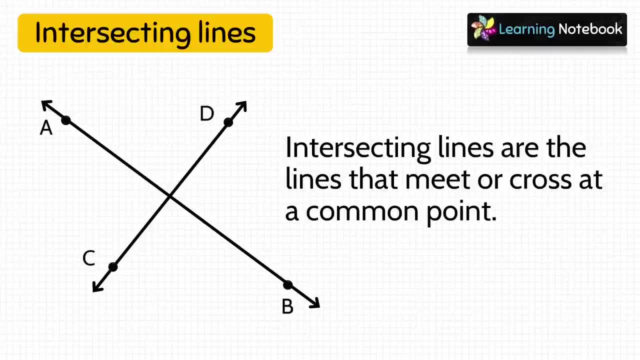 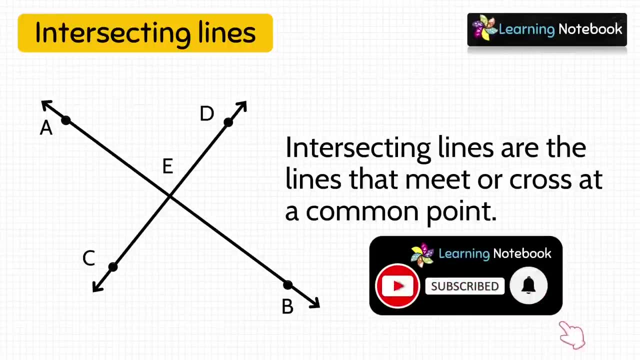 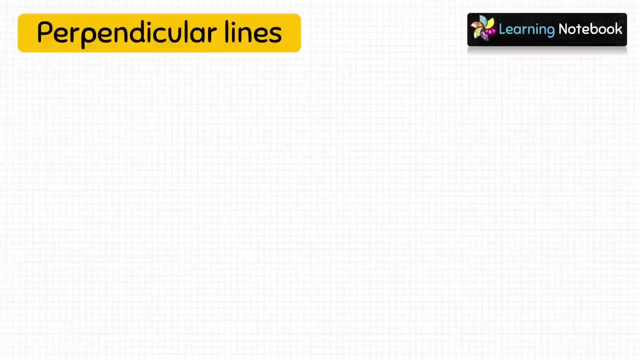 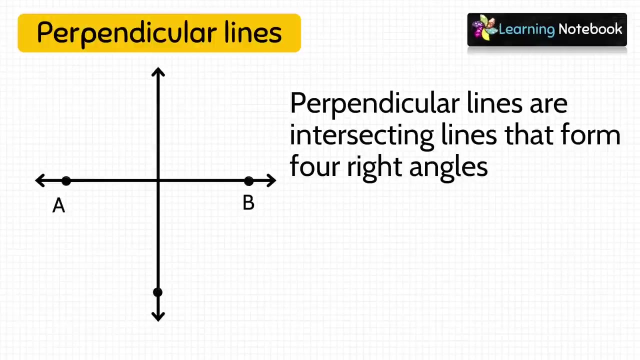 are the lines that meet or cross at a common point. Like here, line AB and line CD are intersecting at a common point E, at a common point E. Next type is Perpendicular Lines. Perpendicular lines are also intersecting lines, but they intersect. 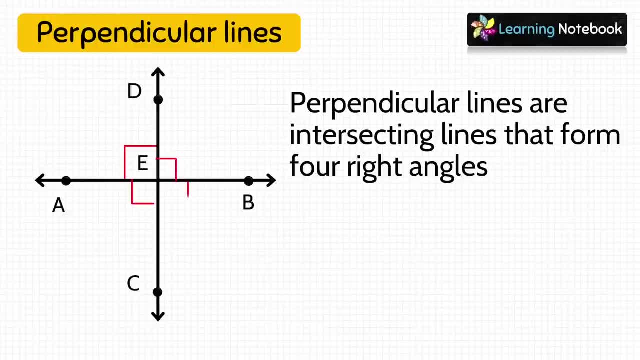 to form four right angles. As you can see here, line CD is perpendicular to line AB and they are intersecting at point E to form four right angles. We have a special symbol to denote perpendicular lines, So we will write: line CD is perpendicular to line AB. 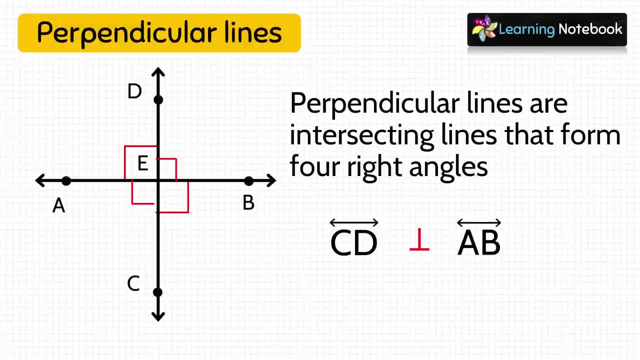 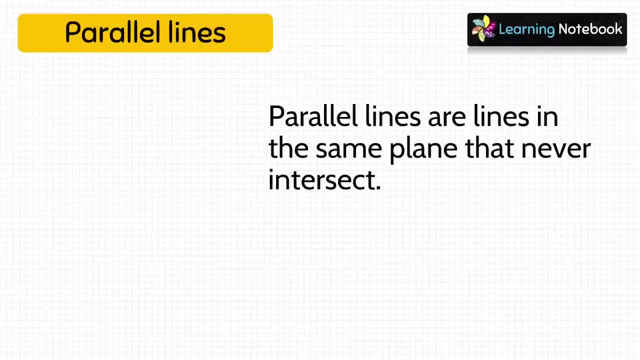 So this is the symbol of perpendicular lines. Now, third type of lines are parallel lines. Parallel lines are lines in the same plane that never intersect. As you can see on the screen, line AB and line CD are parallel lines. They will never intersect each other. 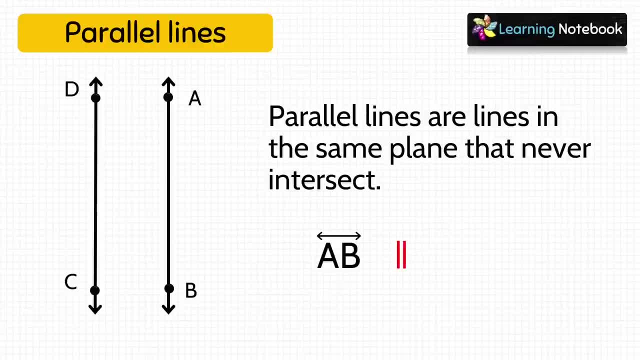 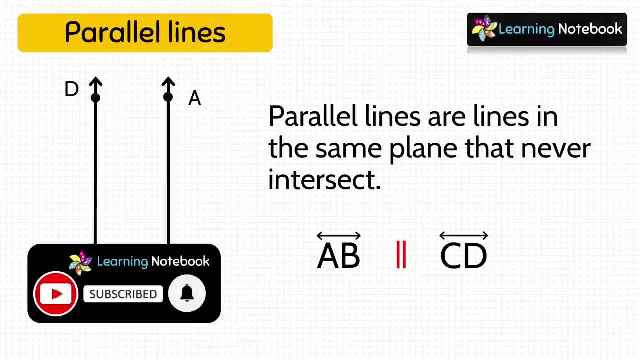 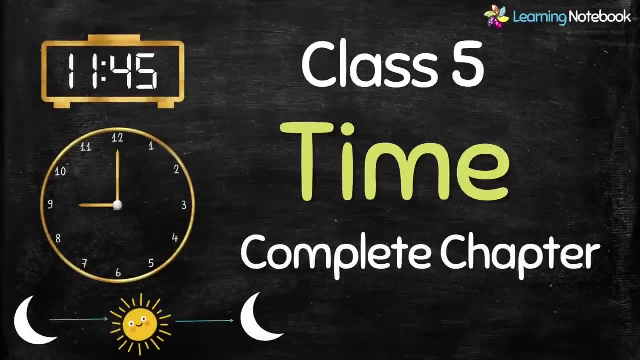 So we will use a special symbol to denote parallel lines. So we will write: line AB is parallel to line CD. So this symbol in red is a symbol of parallel lines. Students, we also have a separate video on chapter time for class 5.. 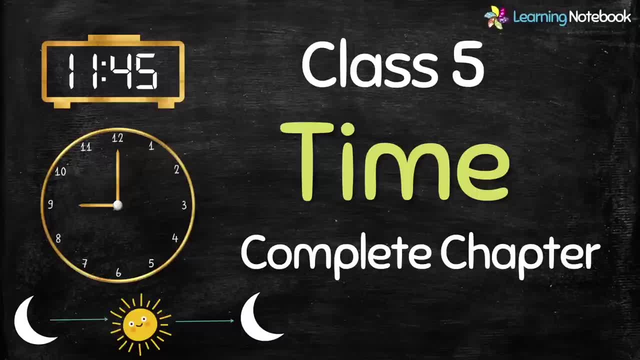 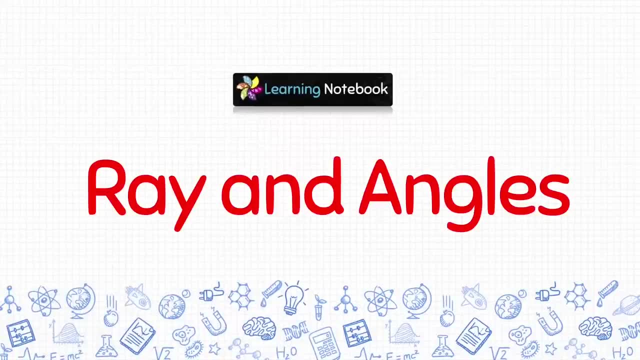 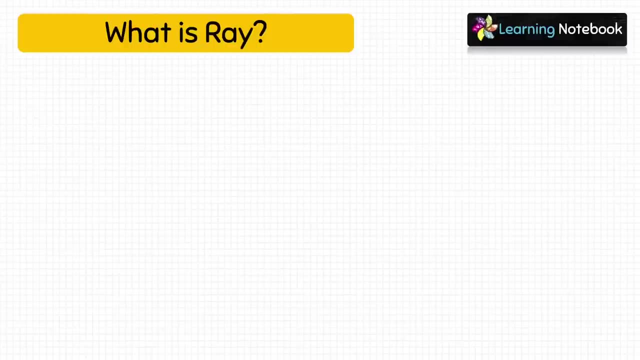 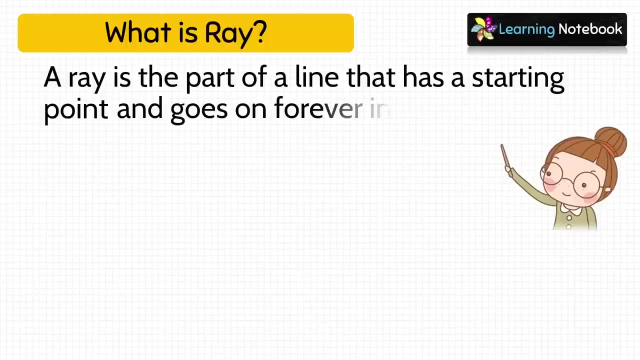 We will talk about time duration of an activity and lot more. So do watch this video Now. next topic is way and angles. First, let's understand what is way. A way is a part of the line that has a starting point and 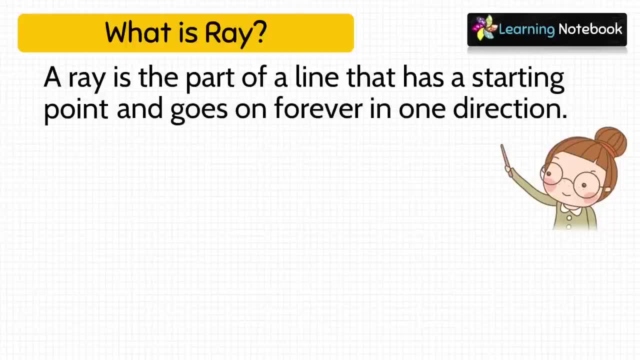 it goes on forever in one direction. Way also has no fixed length. It cannot be measured. For example, this is a ray. It has a starting point called K and it goes indefinitely in one direction, towards J. Now let me show you how to read and write. 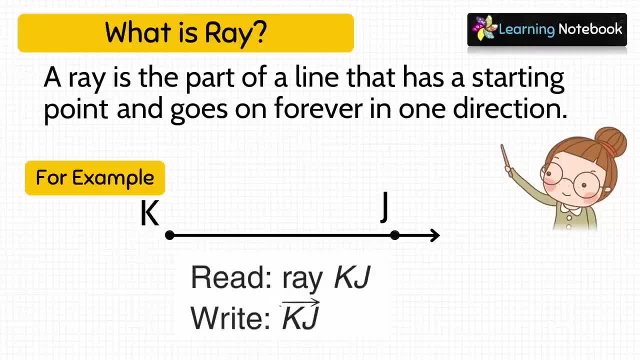 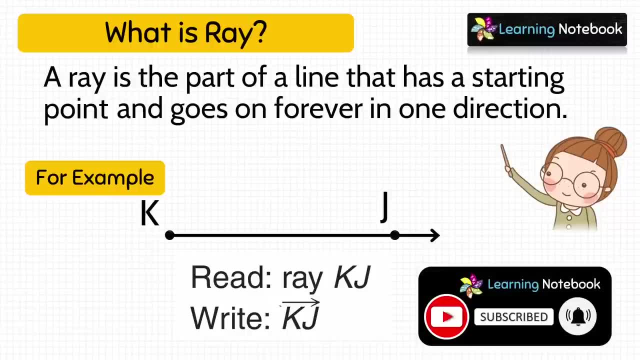 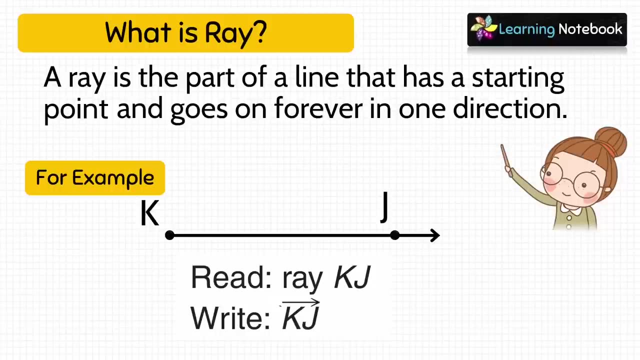 way. We will read the starting point first. So it will be read as way, KJ. Thus, students, there is only one way to read way, That is, by reading the starting point first. And now how to write it. We will write it, KJ. 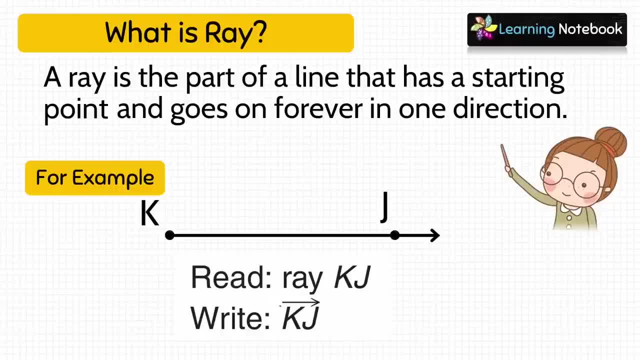 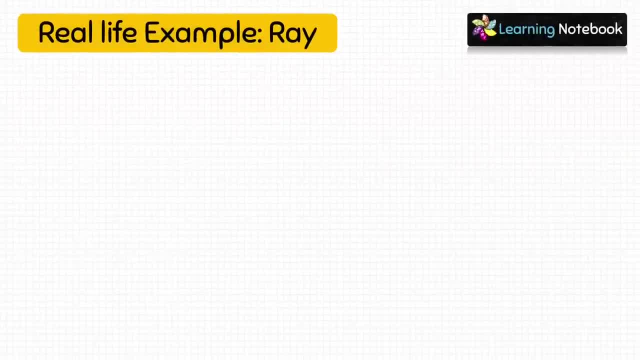 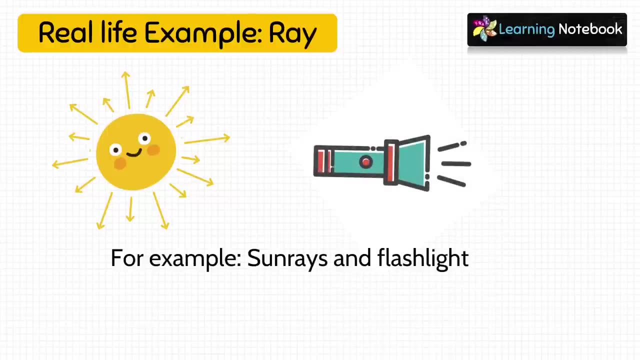 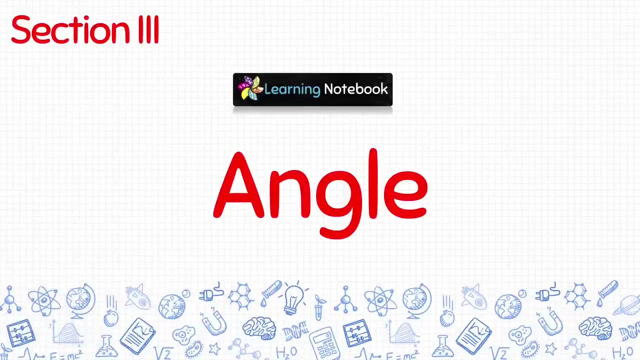 with a small way drawn over it. Now let's see some real life examples of way: Rays from sun and rays from flashlight. These are examples of way Because they have a starting point and they go indefinitely in one direction. Now, in section 3, we will learn. 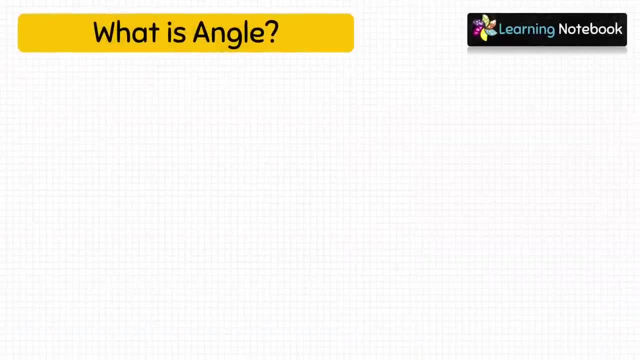 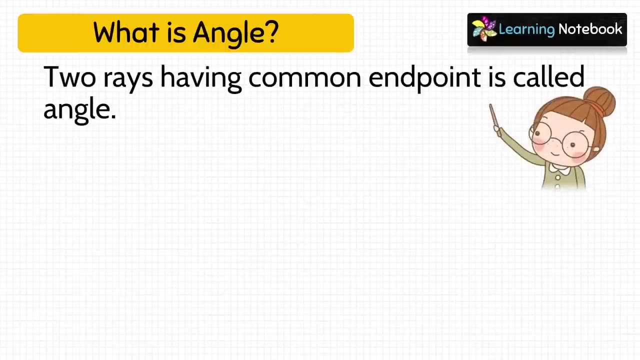 about angles. Two rays having a common end point is called angle. For example, here way AB and way AC are forming an angle. The two rays are called arms of the angle And the common end point is called vertex of the angle. So, students, 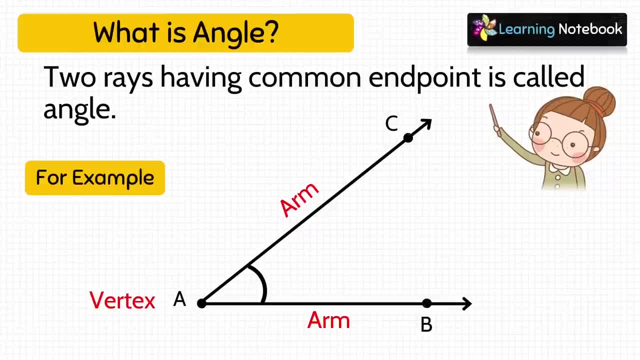 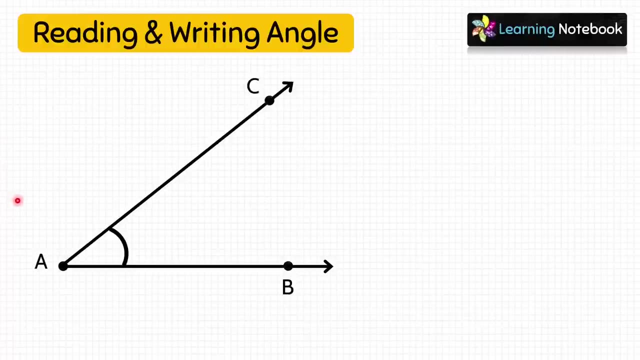 A is the vertex here, while AC and AB are arms of the angle. Now let's learn how to name an angle. To name an angle, we need three points, And the point at which an angle is formed will always be in the middle. 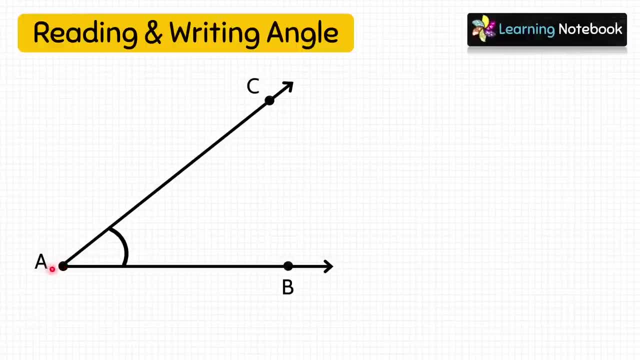 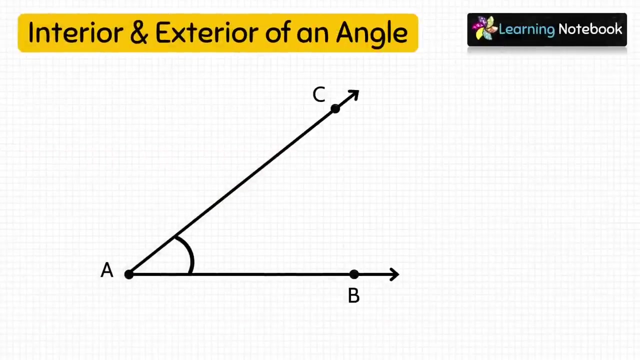 Here angle is formed at vertex A, So A will always be in the middle while naming this angle, So we can read and write this angle as angle A or angle CAB or angle BAC. Now let's see what is interior and exterior of an angle. 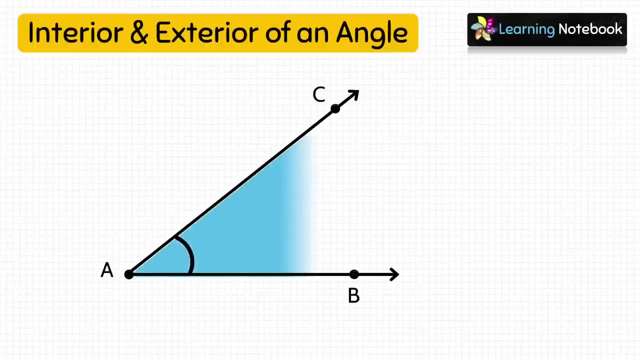 Let's consider an angle CAB. So this shaded region is the interior of angle CAB, While the rest of the area is considered to be exterior of an angle. So let's take a point I. This point lies in the interior of an angle. 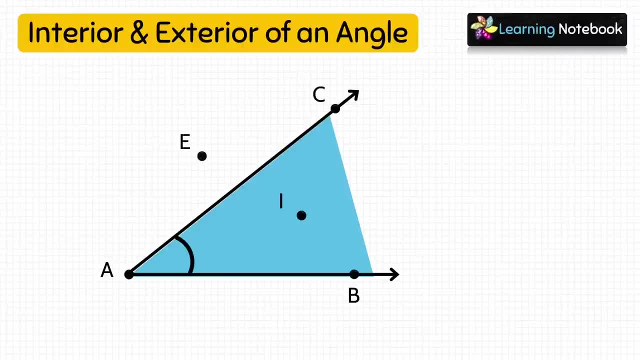 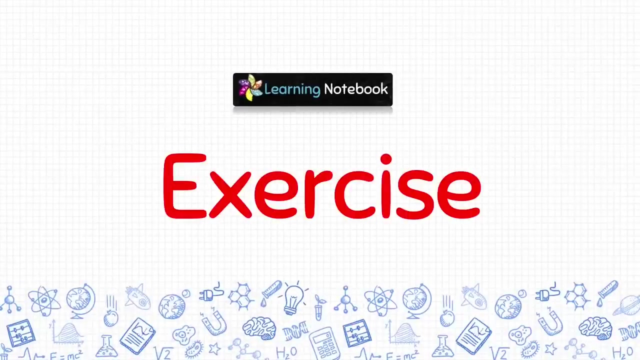 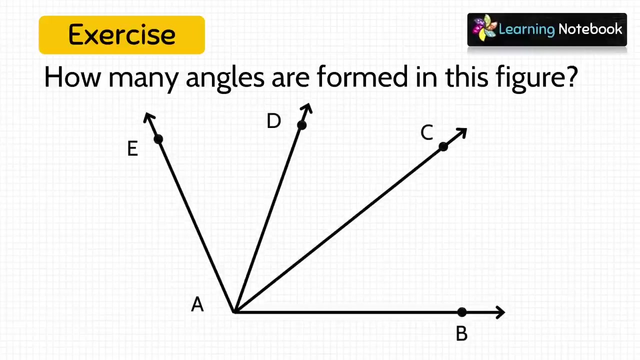 While the point E lies in the exterior of the angle And other points like P and Q, they lie on the angle CAB. Now, to revise these concepts, let's do an exercise. How many angles are formed in this figure? Students look at this. 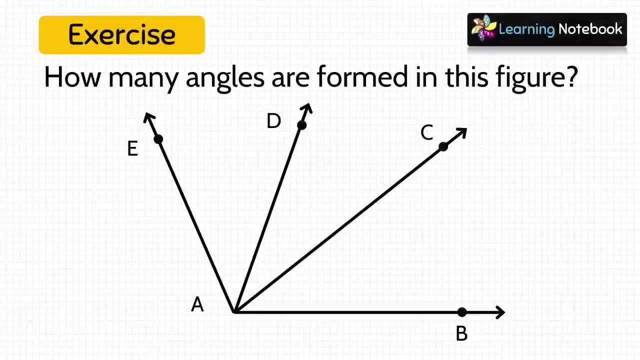 figure carefully. We can see only three angles in this figure or do we have more angles formed in this figure? Let's check it out. First angle which we can see is angle BAC. Second angle being formed here is angle CAD And third angle is: 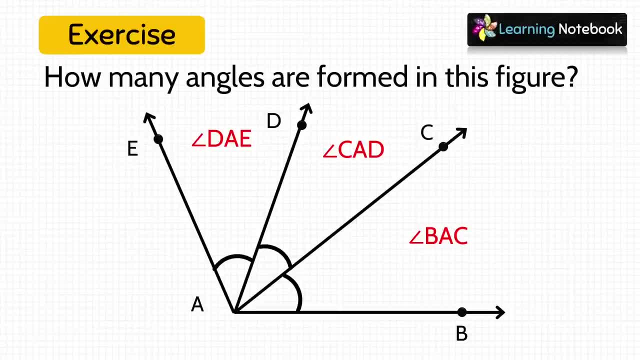 angle DAE. Now look carefully. We have another angle, which is called angle CAE. Then fifth angle being formed here is angle BAD, And last angle being formed here is angle BAE. So it means six angles are being formed in this figure. 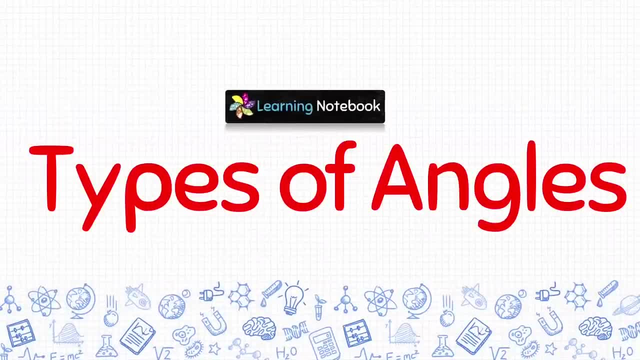 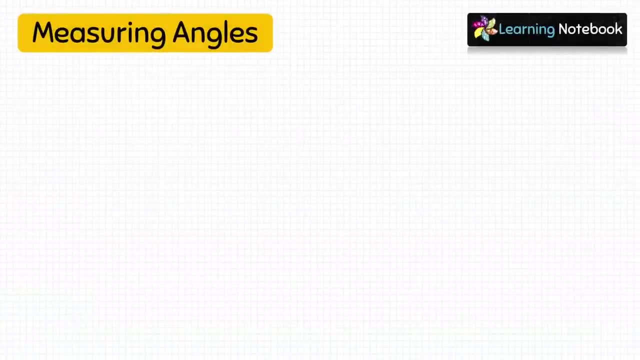 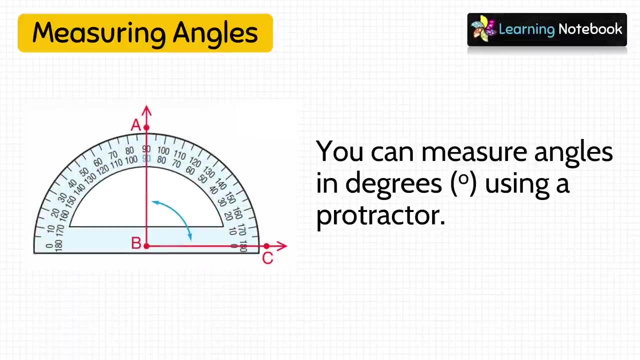 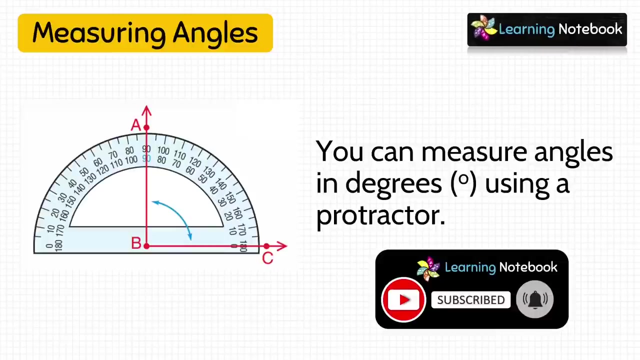 Now let's learn about types of angles. First, let me tell you a little bit about measuring angles. Measure of an angle is the distance between its two arms. You can measure angles in degrees using a protector. We will learn how to measure angles using a protector. 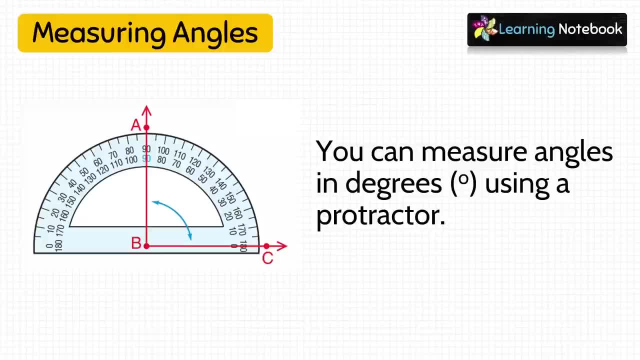 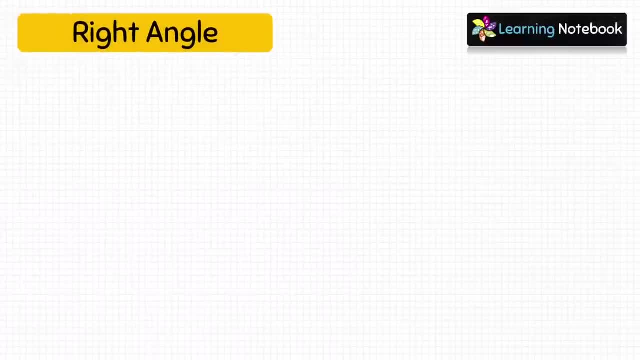 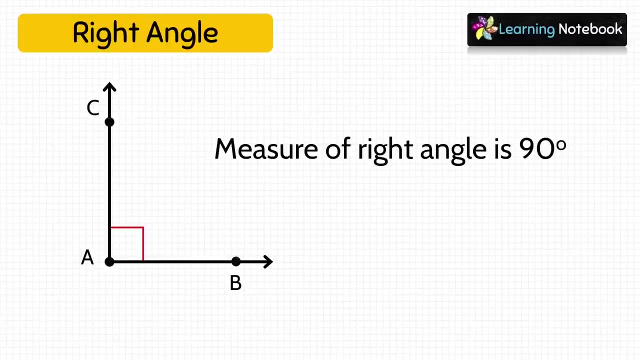 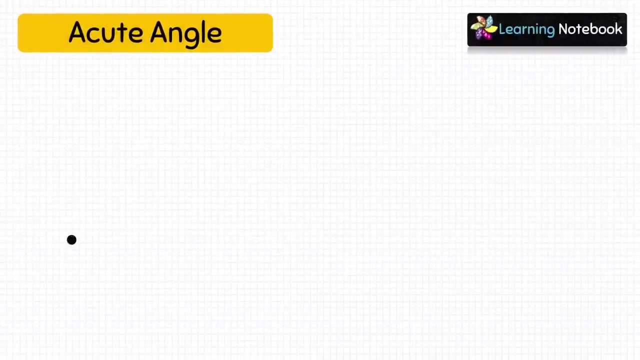 later in the video. But for now you understand that angle is measured in degrees. Now let's learn types of angles. First is right angle. The measure of right angle is 90 degree, as shown here. This is a right angle. Now next type. 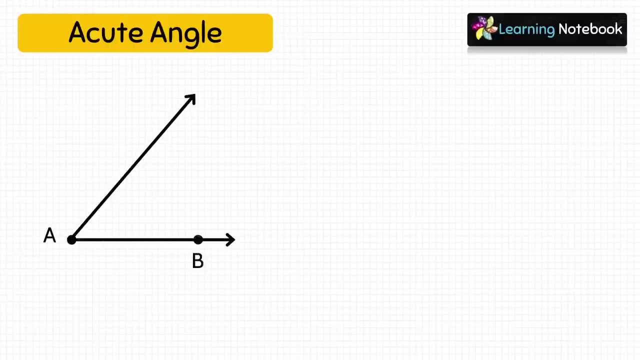 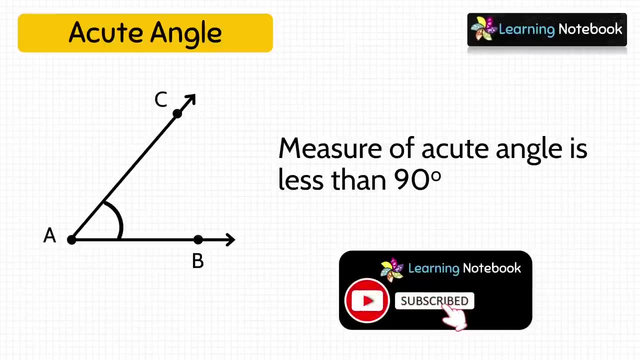 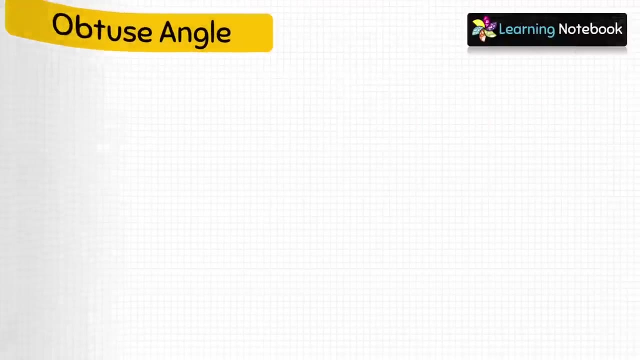 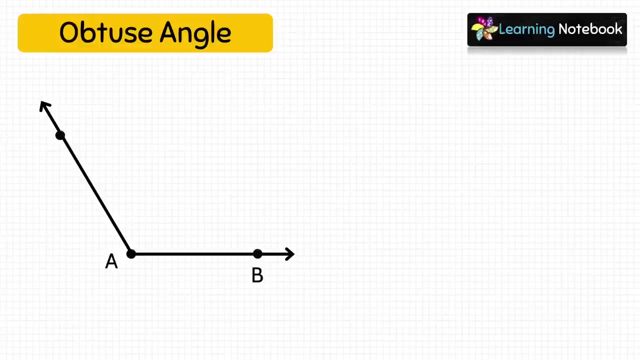 of angle is acute angle. As you can see, this angle measures less than 90 degree. So measure of acute angle is always less than 90 degree. The third type of angle is obtuse angle. Measure of obtuse angle is more than 90 degree. 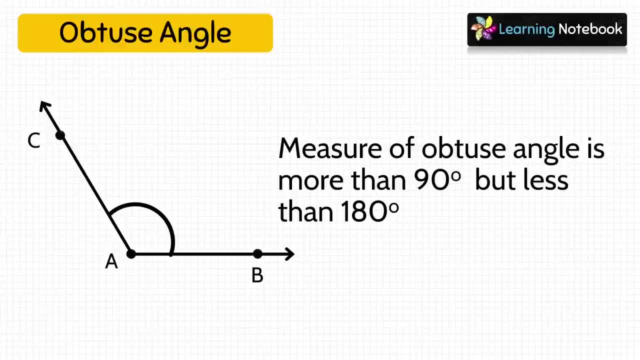 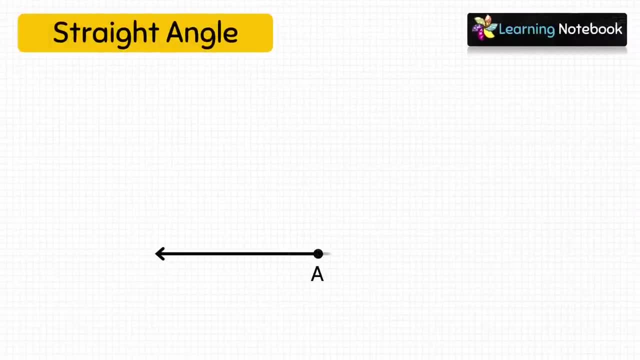 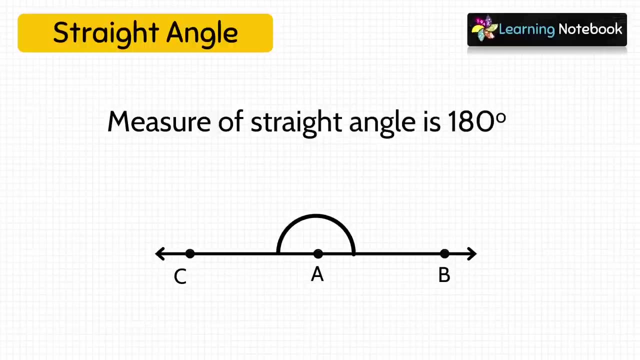 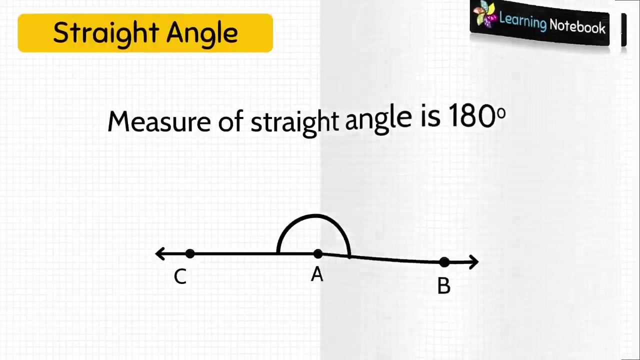 but less than 180 degree. Next type of angle is straight angle. Measure of straight angle is exactly 180 degree, Like here in the given figure. angle CAB is a straight angle because it measures exactly 180 degree. Next is reflex angle. 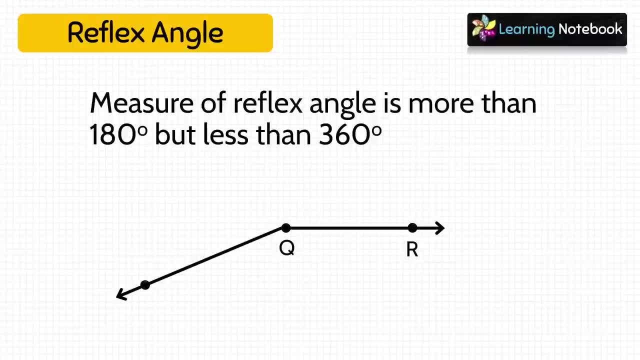 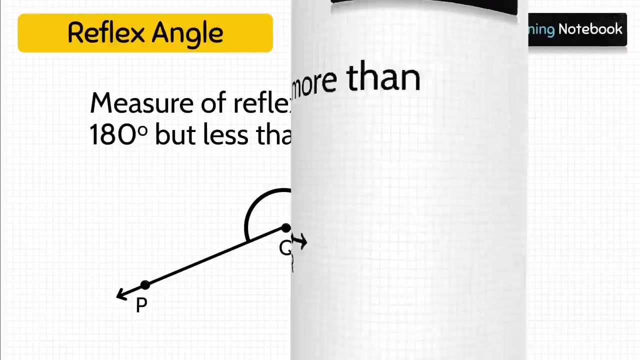 Measure of reflex angle is more than 180 degree but less than 360 degree, Like here in the given figure, angle PQR is more than 180 degree but less than 360 degree. So angle PQR is a reflex angle And the last type of angle 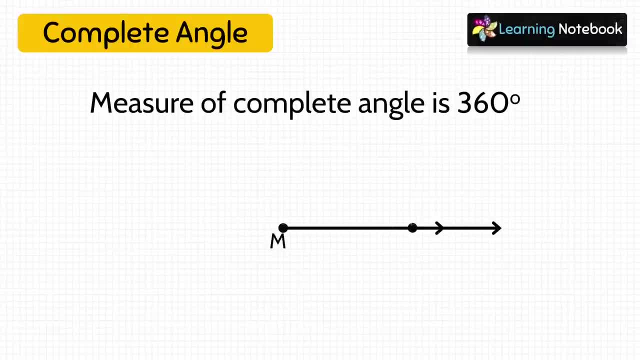 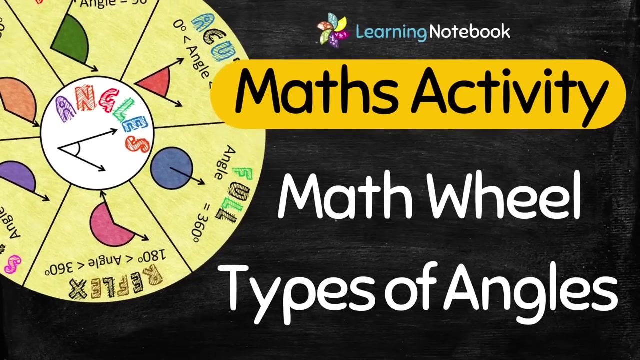 is complete angle. Measure of complete angle is exactly 360 degree, Like here. angle LMN equals to 360 degree. Therefore, angle LMN is a complete angle. Students, it is always fun to learn maths through activities, So we have got a very 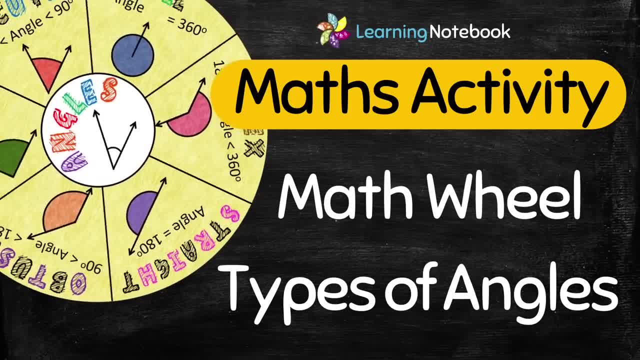 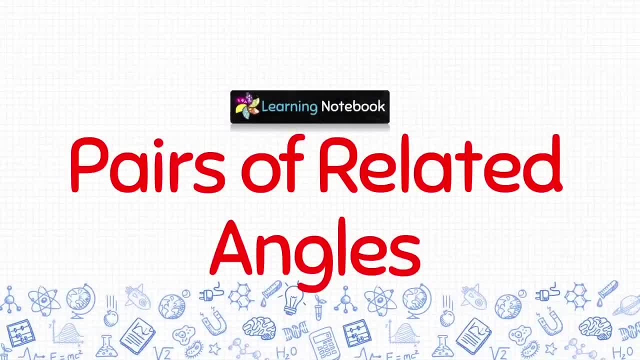 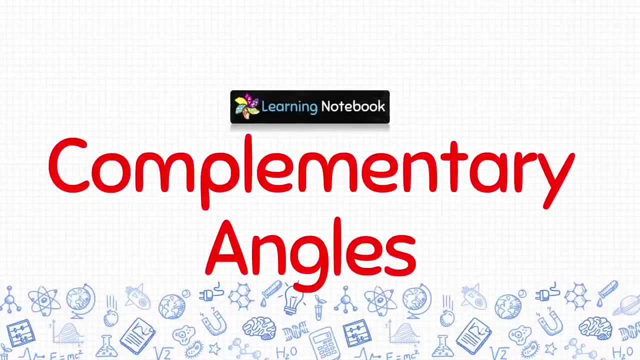 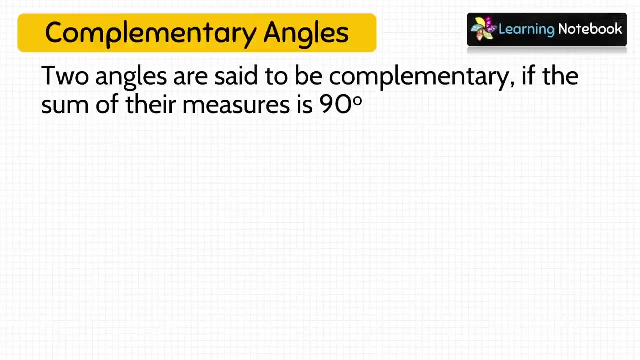 interesting activity for you on types of angles. Do watch this video Now. next topic is pairs of related angles. First type is complementary angles. So what are complementary angles? Two angles are said to be complementary if the sum of their measures is 90 degree. 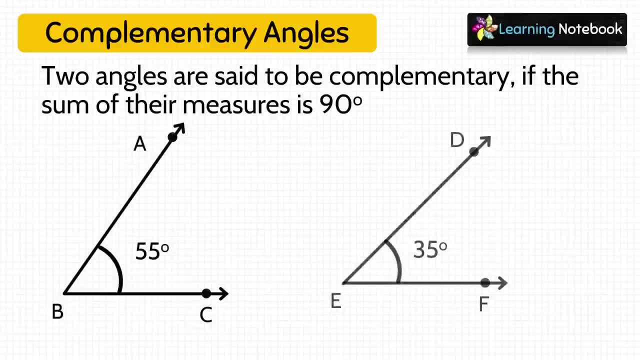 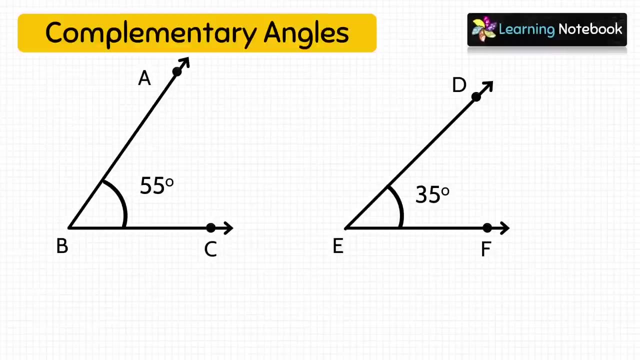 For this, let's consider two angles: angle ABC and angle DEF. They measure 55 degree and 35 degree respectively. Now if we add the measure of both these angles, that is, 55 degree plus 35 degree, we get 90 degree. 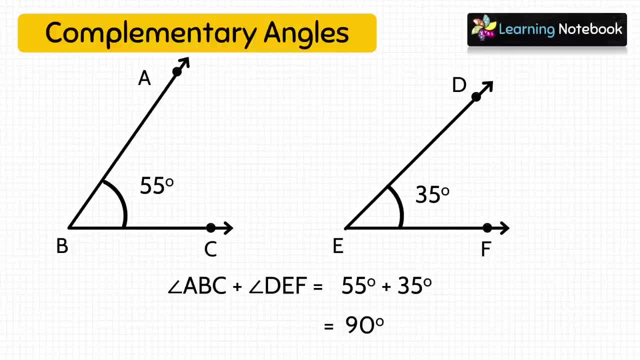 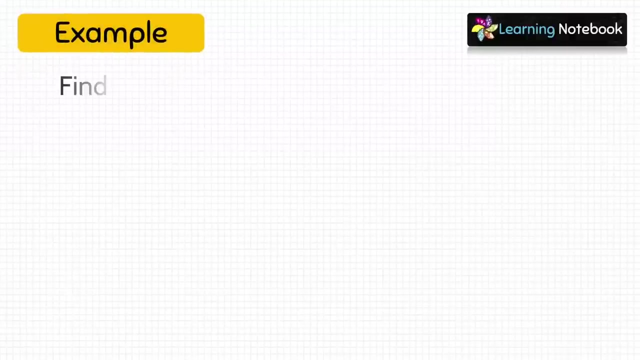 So it means angle ABC and angle DEF are complementary angles because the sum of their measures is 90 degree. Also, we can say that each one of these angles is the complement of the other angle. Now let's do a related question: Find the complement. 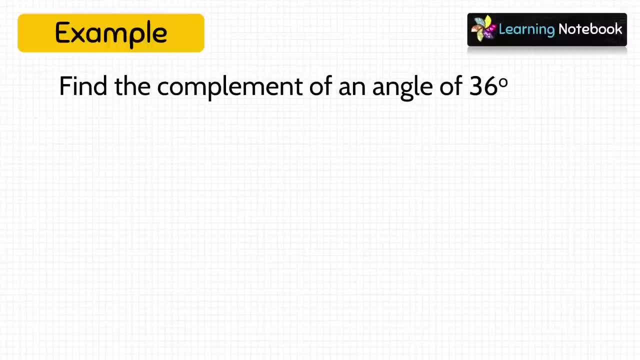 of an angle of 36 degree. So here we have to find the second angle, such that sum of both these angles is 90 degree. So it would be 90 minus 36, which is equals to 54 degree. So complement of 36 degree. 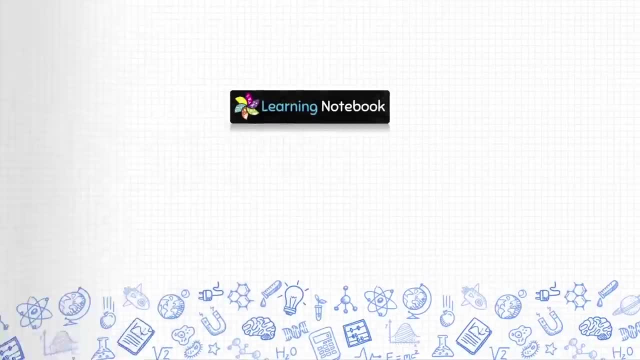 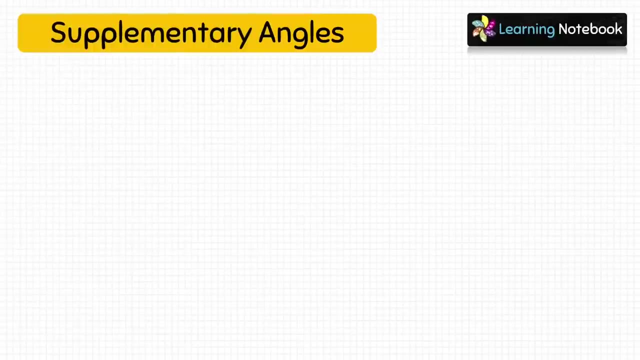 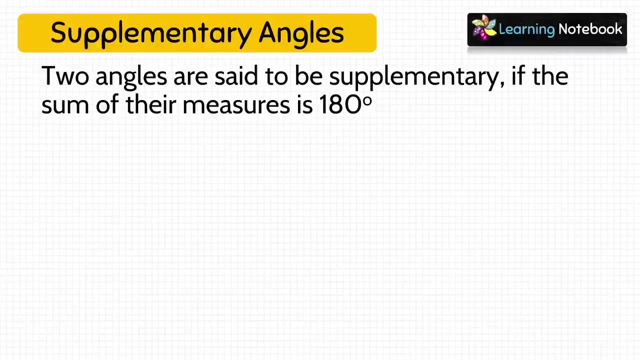 is 54 degree. Now, next is supplementary angles. Two angles are said to be supplementary if the sum of their measures is 180 degree. Again, let's consider either two angles, ABC and DEF. This time they measure 130 degree and 50 degree. 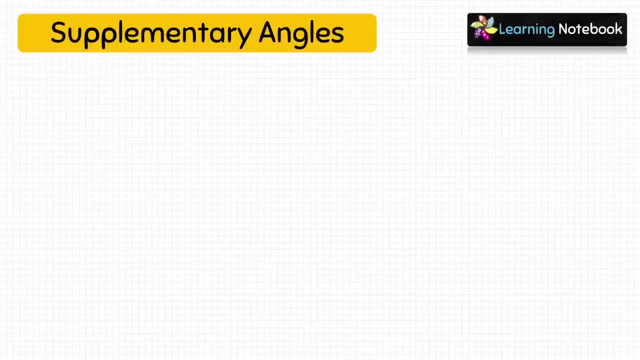 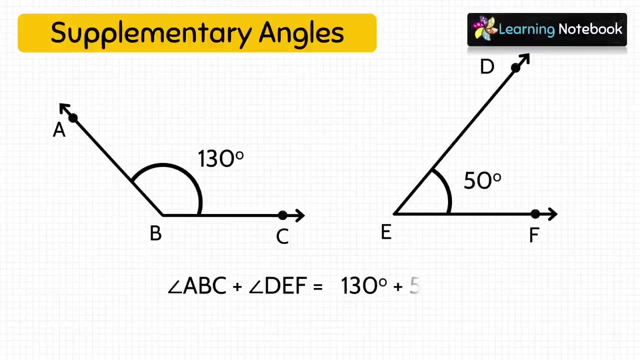 respectively. Now if we add the measures of both these angles- that is, 130 plus 50, we get the measure as 180 degree. So both these angles are supplementary angles because the sum of their measure is 180 degree. We can also say that angle. 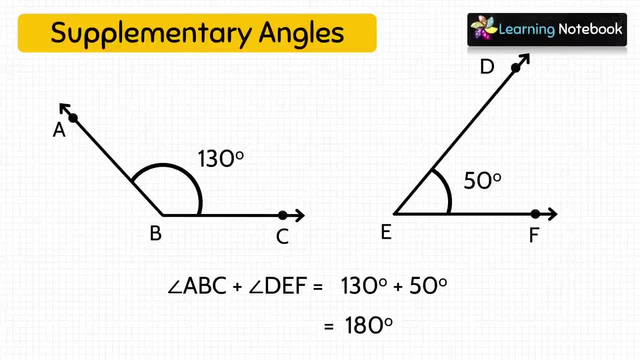 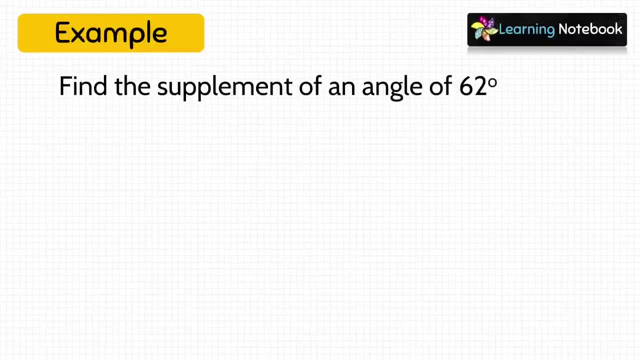 ABC and angle DEF are supplement of each other. Now let's do a related question. Find the supplement of an angle of 62 degree. So here we have to find the second angle, such that sum of both these angles is 180 degree. So 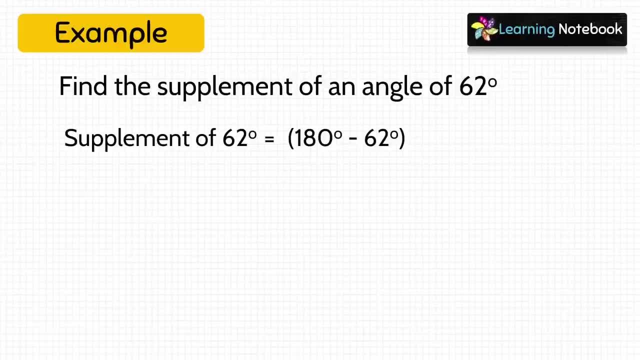 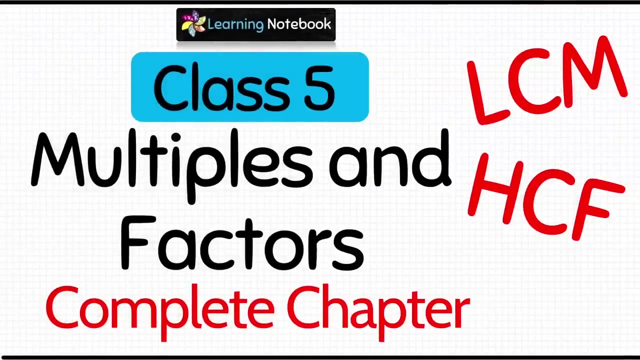 supplement of 62 degree would be 180 minus 62, which is equals to 118 degree. So we will write the answer as: supplement of 62 degree is 118 degree. Students, we have a separate video on chapter multiples and factors for class 5.. 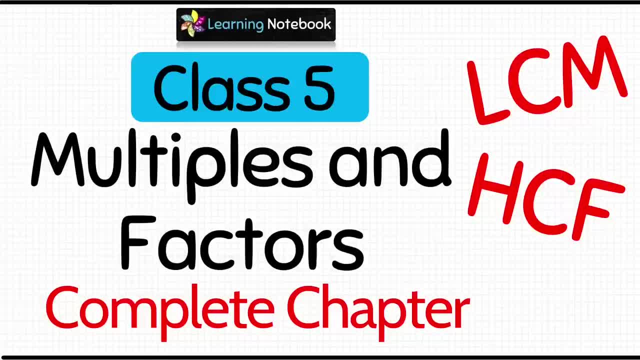 Here you can learn about factors, multiples, their properties, divisibility of numbers, prime and composite numbers, prime factorization, highest common factor and least common multiple. I am sure you would find this video very useful for you. Now let's see how to measure angles. 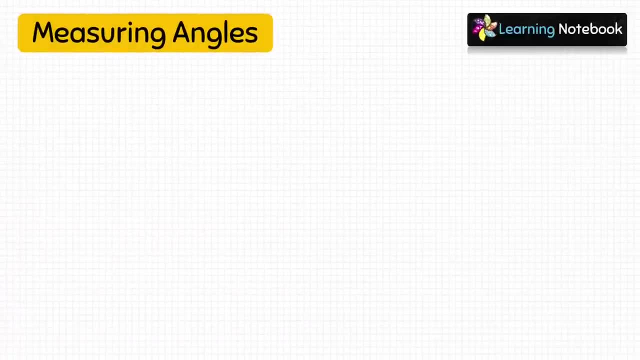 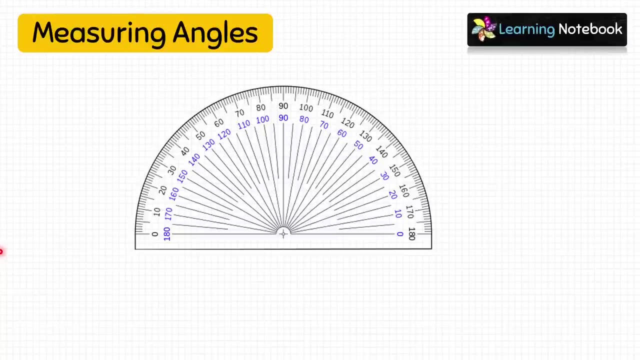 Earlier in the video, I told you that to measure angles we use an instrument called a protector. So this is the protector I was referring to. A protector has two edges: One is semi-circular edge and the other is this straight edge. The straight edge has: 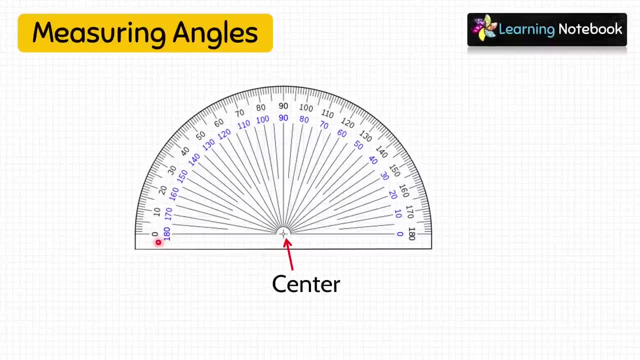 a centre and a base line. Now the semi-circular edge is marked with 0 to 180 degrees clockwise as well as anti-clockwise. Numbers in black are written clockwise and they are called as outer scale, While numbers in blue are written anti-clockwise. 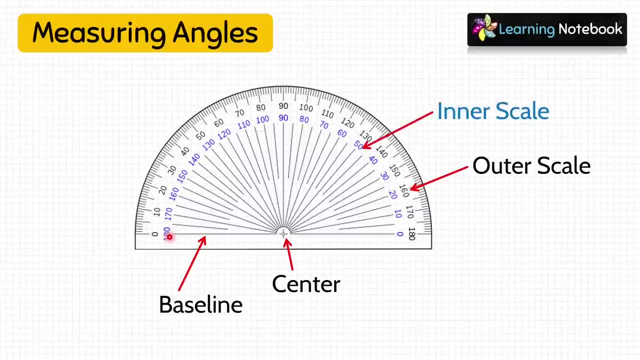 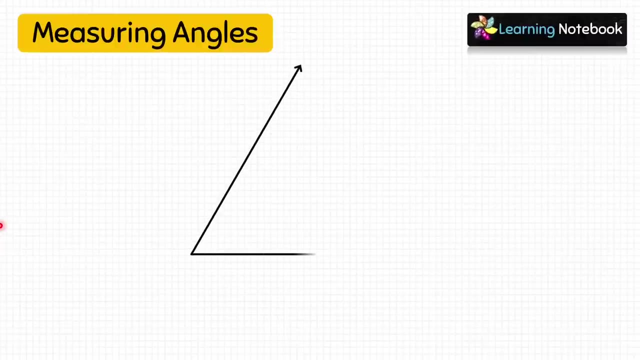 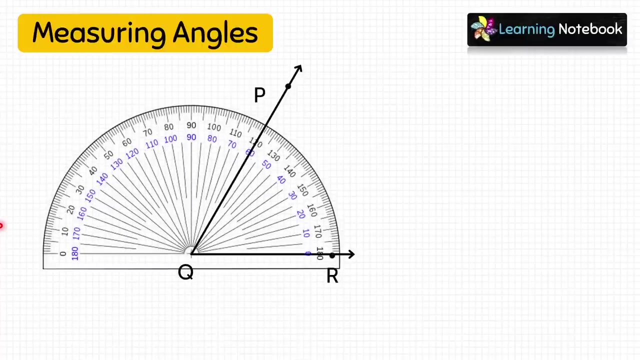 and they are called as inner scale And degree, is the unit of measuring angles. Now let's see how to use this protector to measure a given angle. Here we have to measure the angle PQR. So first let's place the base line of the protector on. 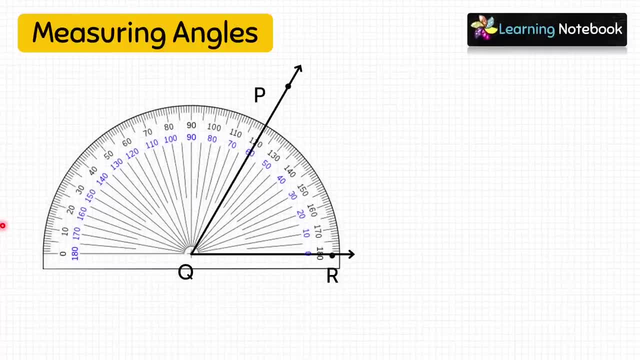 the arm QR of the angle, such that the centre of the protector is on vertex Q. Now students check where is 0 degree, because we have to start from 0.. As you can see, 0 degree is on inner scale, So we will use. 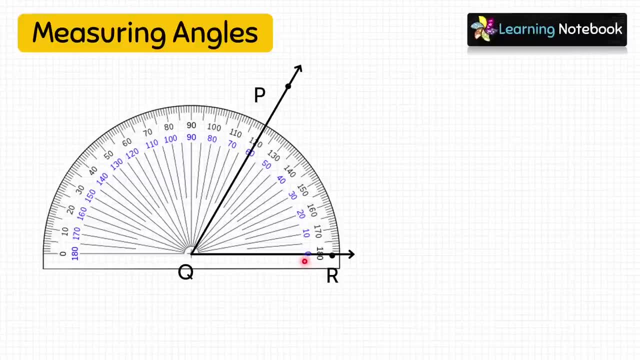 inner scale to measure this angle. Now check the other arm, QP. It crosses the inner scale on the protector at 60 degree. So the measure of angle PQR is 60 degree. We will write it as angle PQR equals to 60 degrees. 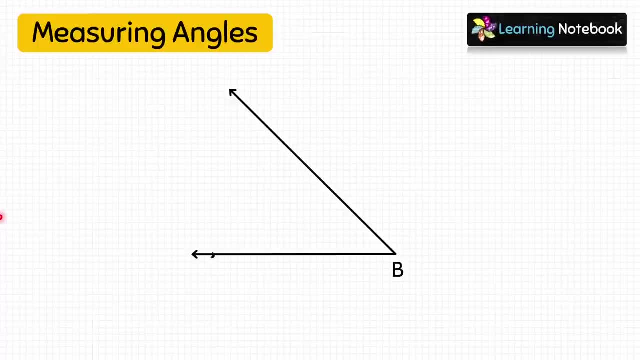 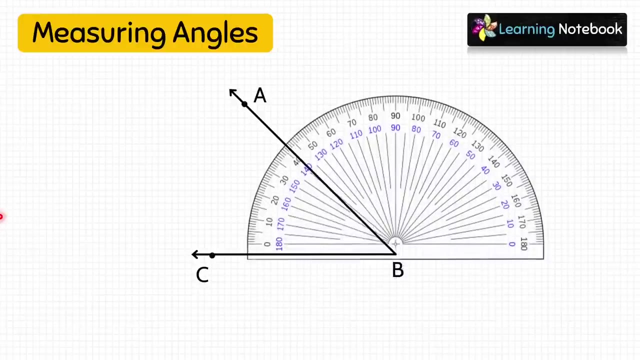 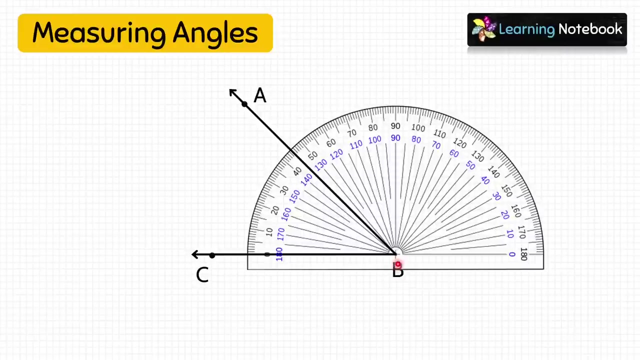 Now, students, let's see how to use the protector if the base line is in the opposite direction. Here we have to measure this angle ABC. So first let's place the base line of the protector on the arm BC, such that the centre of the protector is on vertex. 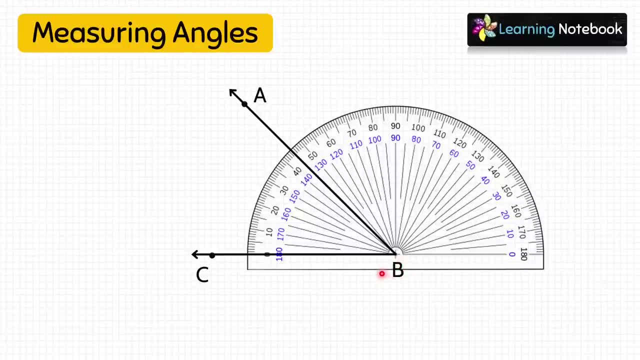 B. Now check where is 0 degree. 0 degree is on outer scale this time, So we have to use outer scale to measure this given angle. Now check the other arm AB. It crosses the outer scale on the protector at 45 degree. 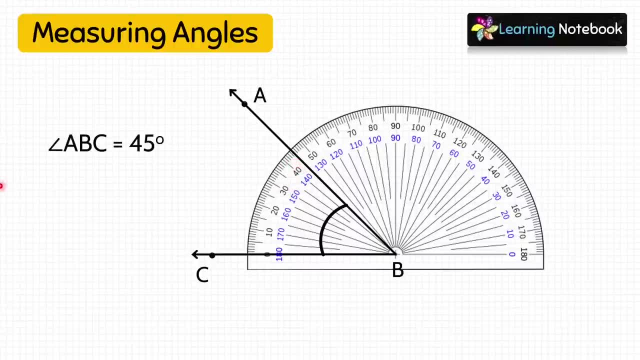 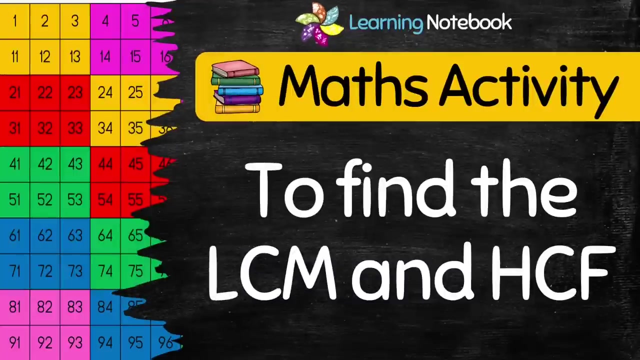 So the measure of this angle ABC is 45 degree. We will write: angle ABC equals to 45 degrees. So, students, in this way you can use protector to measure any given angle. Students, if you want to learn how to find the least common multiple and 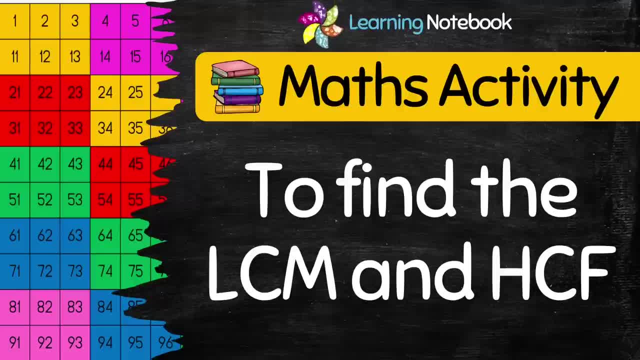 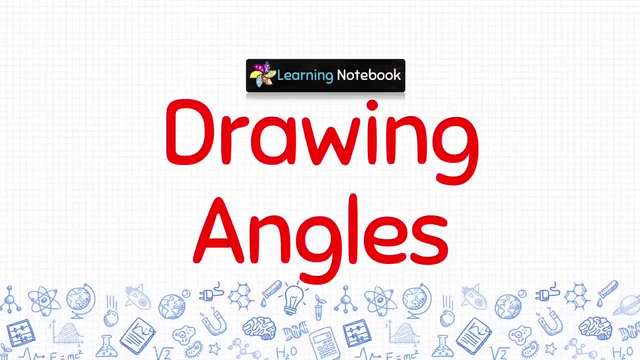 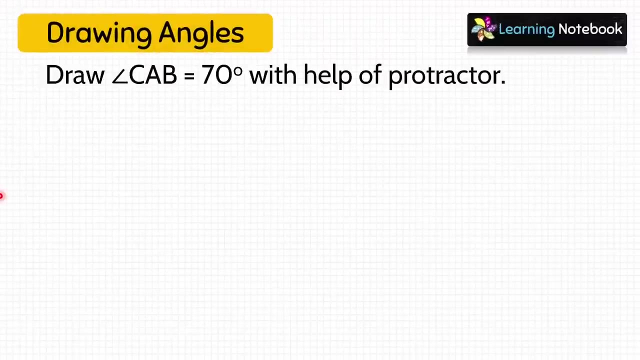 highest common factor with the help of an interesting activity. then do watch this separate video. The link to this video is below in the description box. Now let's continue and see how to draw angles. Question is: draw angle- CAB equals to 70 degree- with the help of a 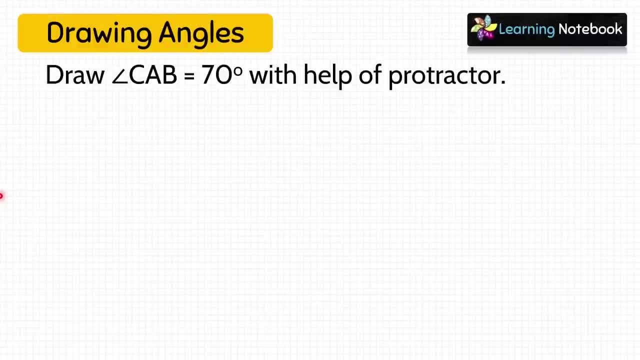 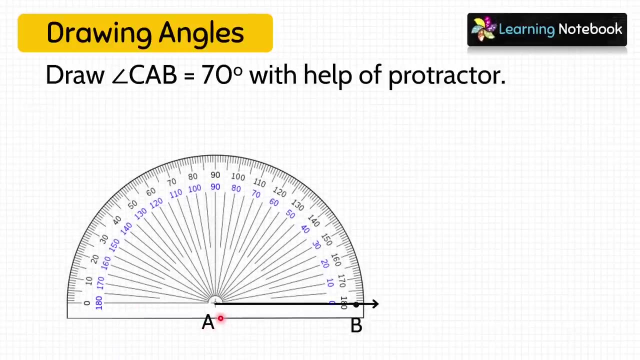 protector. So first draw a line, segment AB. Then keep the base line of the protector on AB with the center at A. Now start with 0 degree and mark a dot at 70 degree and name it C. Now students remove the protector and draw a line. 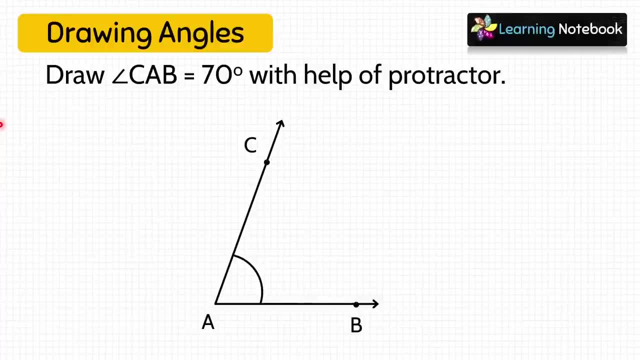 segment joining point C to A. So we have drawn angle CAB equals to 70 degree. Now next question is draw angle CAB equals to 115 degree with the help of a protector. Again, first let's draw a line, segment AB. Next keep the base line. 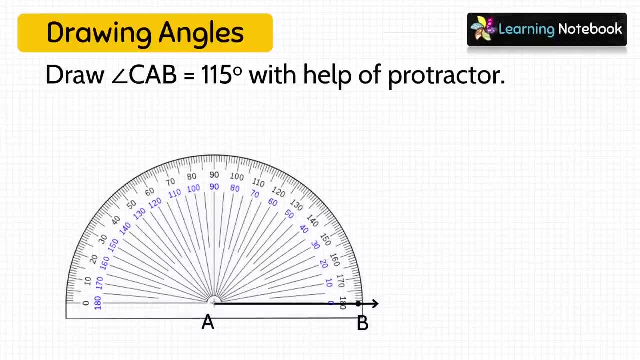 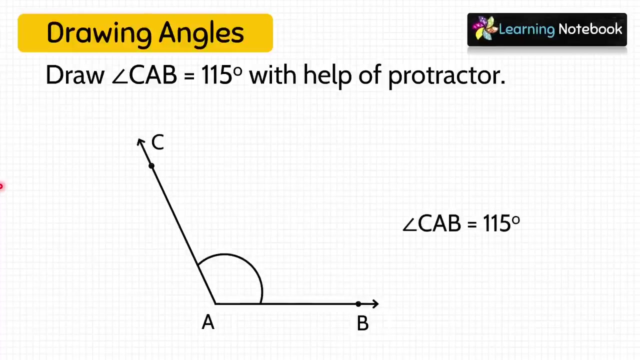 of the protector on AB with the center at A. Now start with 0 degree and mark a dot at 115 degree and name it C. Now remove the protector and draw a line, segment AB, joining point C to A. So we have drawn angle CAB. 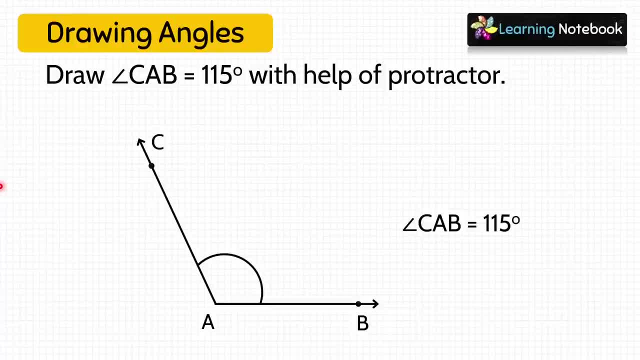 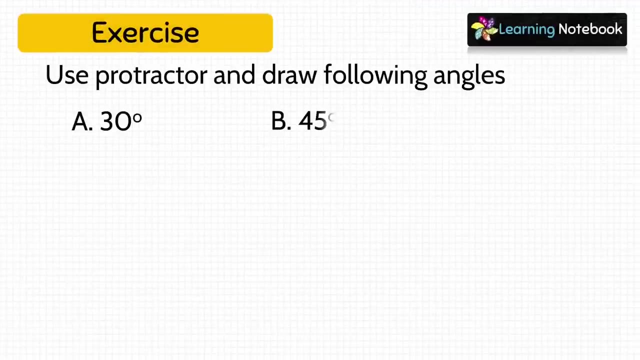 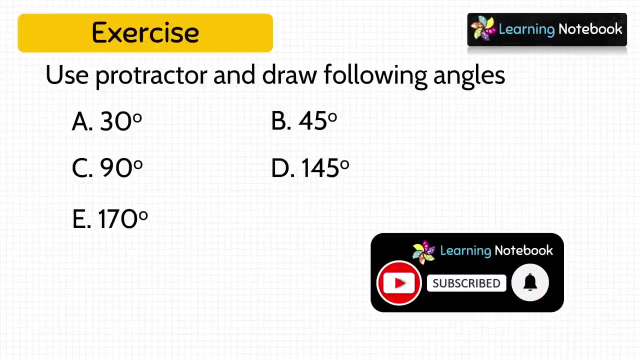 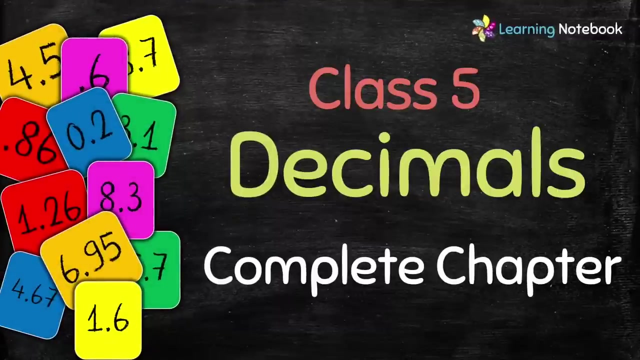 equals to 115 degree. So, students, we have learnt how to draw acute angle as well as obtuse angle with the help of a protector. Now, students, this is practice exercise for you. Use the protector and draw the following angles. We have a separate. 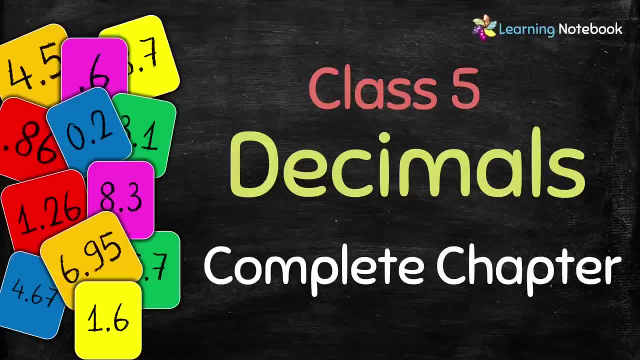 video on complete chapter of decimals for class 5.. Here you can learn about like and unlike decimals, addition of decimals, their subtraction, multiplication and division, as well as how to convert decimals into fractions and vice versa. You will find this video very useful to learn about decimals. 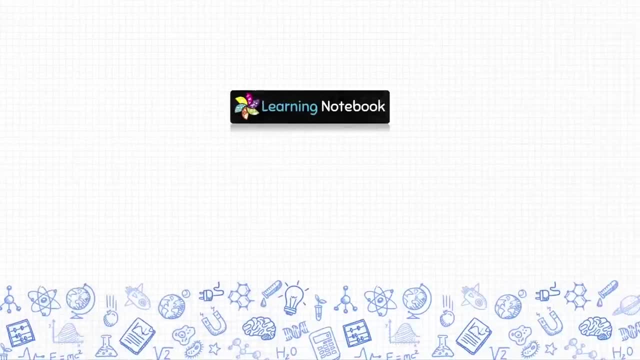 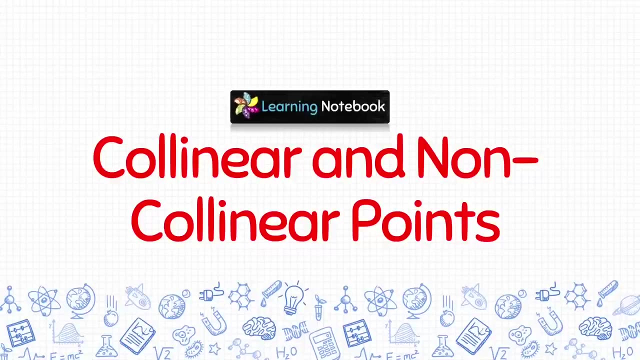 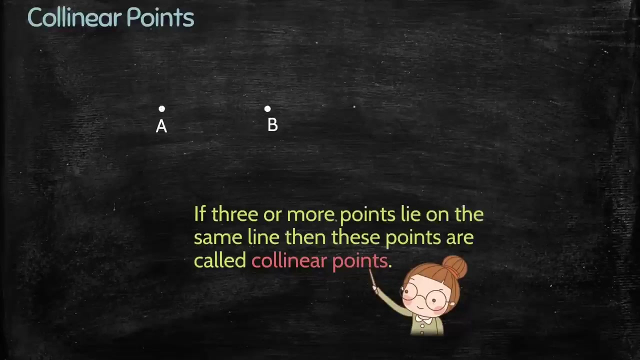 in a comprehensive way. Now let's continue. our next topic is collinear and non-collinear points. First let's see what are collinear points. If three or more points lie on the same line, then these points are called collinear points. 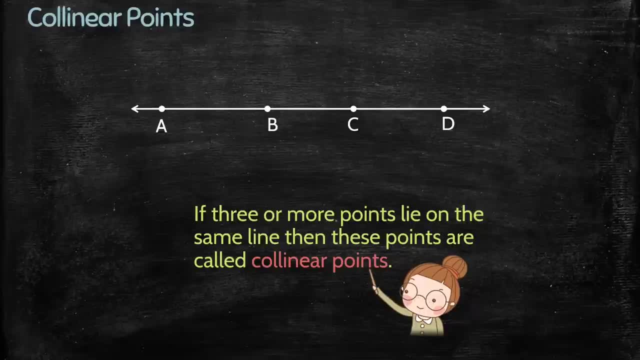 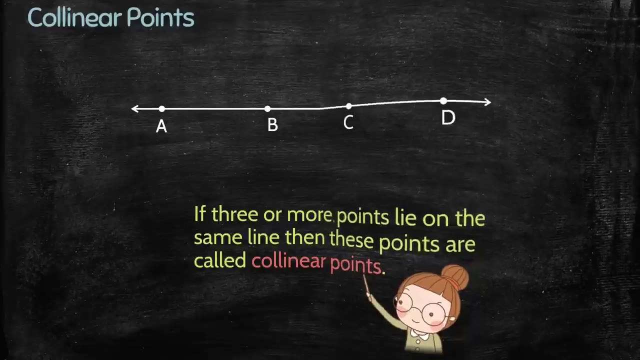 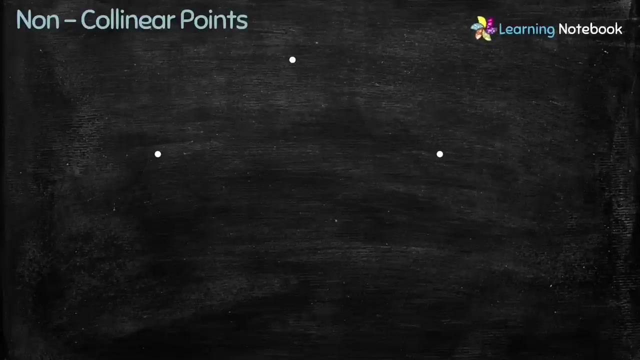 Like here, in the given figure, all the four points A, B, C and D lie on the same straight line. Hence the points A, B, C and D are collinear points. Now look at these three points. If we join them, we will find that these: 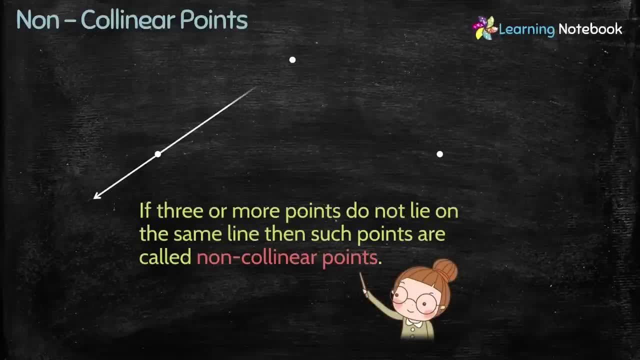 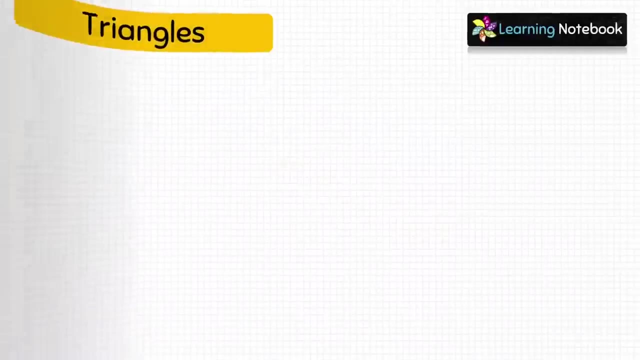 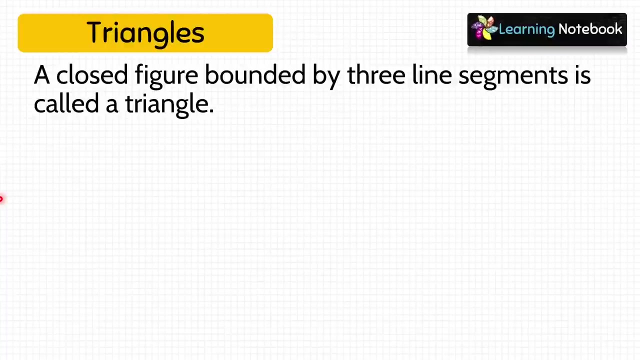 points do not lie on the same straight line, So such points are called non-collinear points. Our next topic is triangles. So what is a triangle? A closed figure bounded by three line segments is called a triangle. Like this closed figure is the. 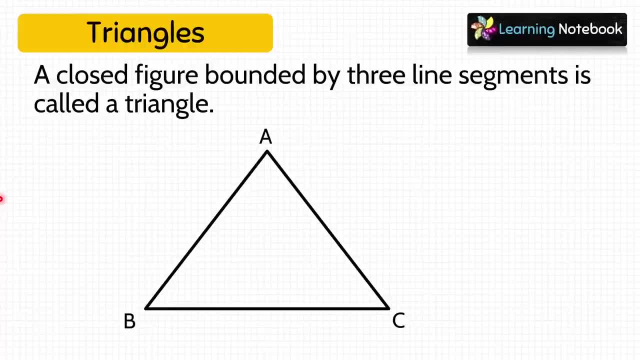 triangle ABC And we write it as like this: This is the symbol of triangle, So we will write triangle ABC. And this triangle ABC has three vertices: A, B and C. It has three sides: AB, BC and C- CA. This triangle ABC has three. 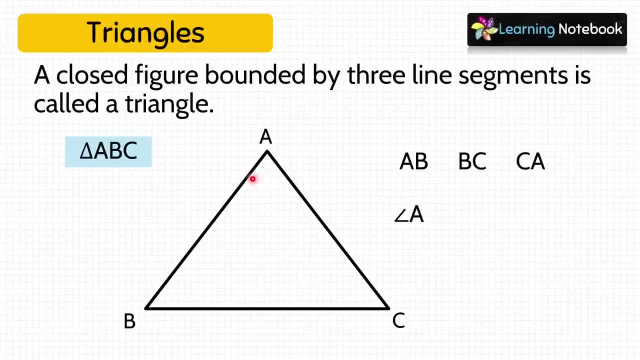 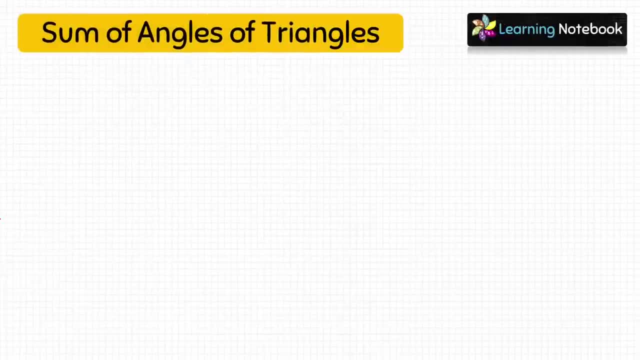 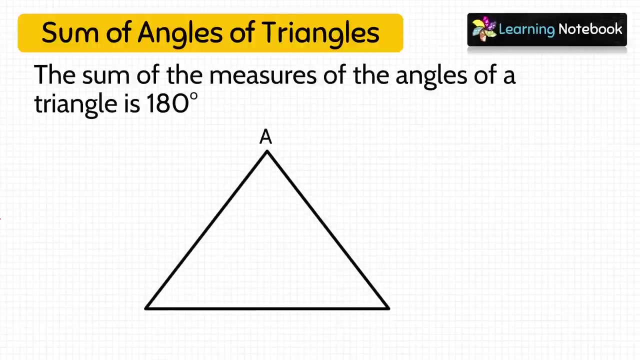 angles: Angle A, angle B and angle C. Now, a very important property of triangles is angle sum property. It says that some of the measures of the angles of a triangle is always 180 degree. It means in the given triangle, ABC, angle A. 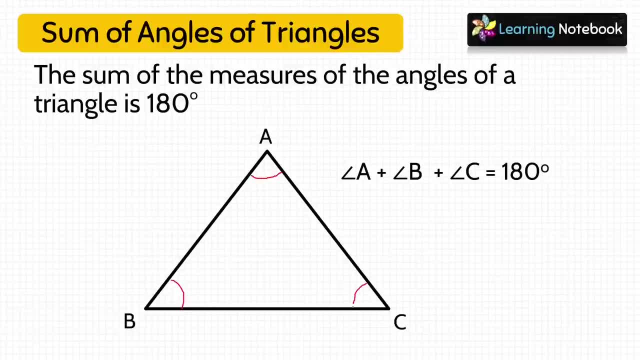 plus angle B plus angle C equals to 180 degree. So, students, this property is very useful while solving some questions. Like you would be given the angles, the measures of the two angles, and you have to find the measure of third angle. So such questions. 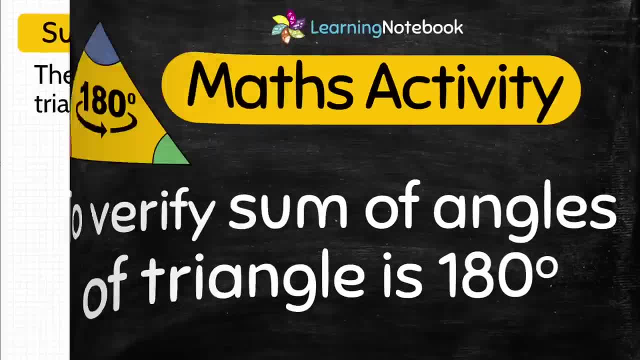 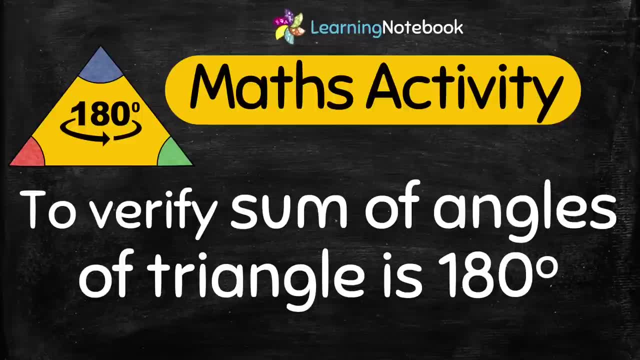 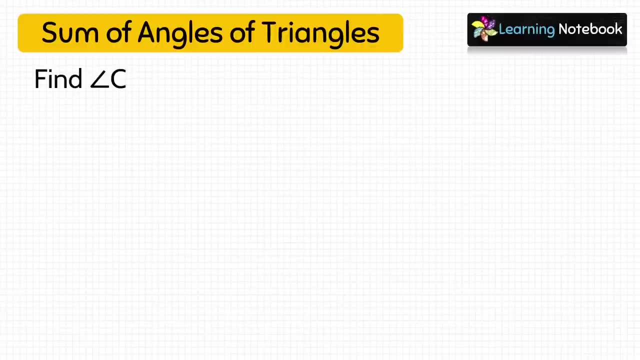 are solved using this property. We also have a related activity to verify this angle sum property. I would recommend you to watch this video. Now let's do a question related to this angle sum property. In the given triangle ABC, we are given with two angles, A and B. 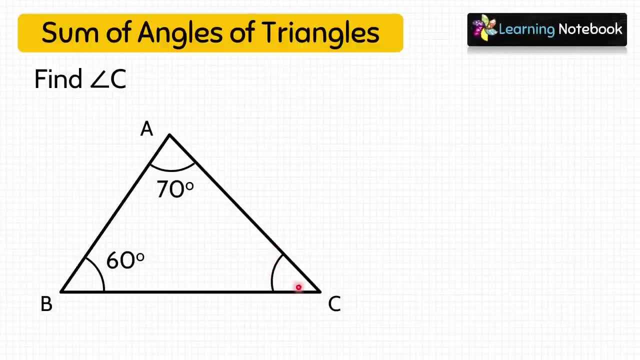 and we have to find measure of angle C. So we just learnt that, according to angle sum property, angle A plus angle B plus angle C equals to 180 degree. Here put the values of angle A and angle B, which is 70 degree and 60 degree. 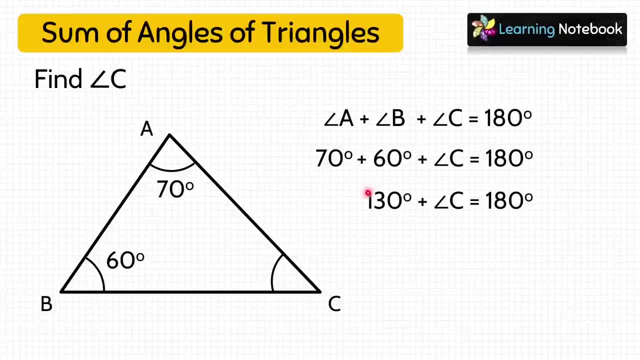 Now add these two values, we get 130 degree. So angle C would be equals to 180 minus 130, which is equals to 50 degree. So this is how we can find the third angle when we are given with the measure of two angles. 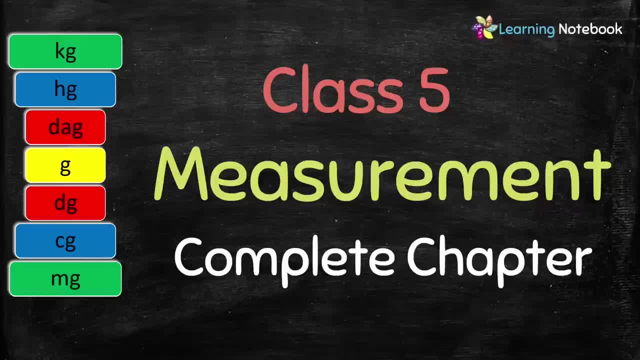 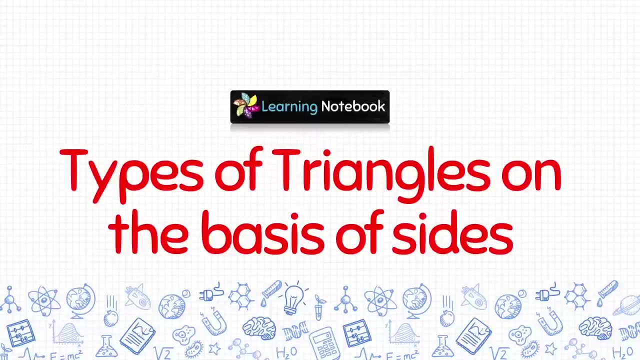 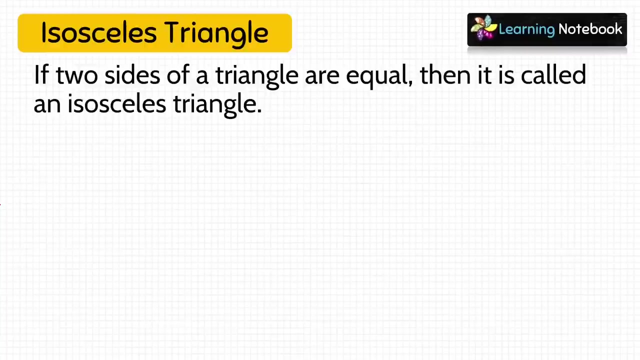 We also have a video on complete chapter of measurement for class 5.. In this video you can learn about measurement of length, mass and capacity. Now let's understand types of triangles on the basis of sides. First type of triangle is isosceles triangle. 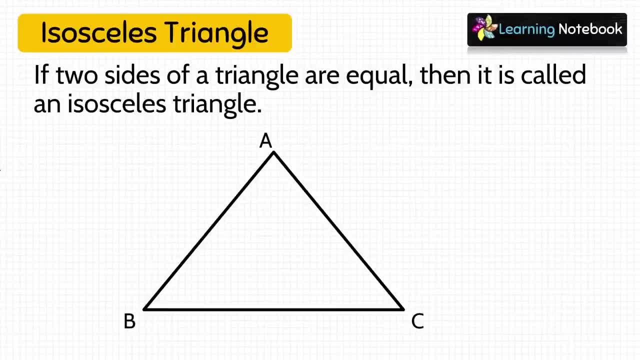 If two sides of a triangle are equal then it is called an isosceles triangle. Like in this triangle, ABC, AB equals to AC, So triangle ABC is an isosceles triangle. Another point to note here is that the angles opposite to the equal sides of 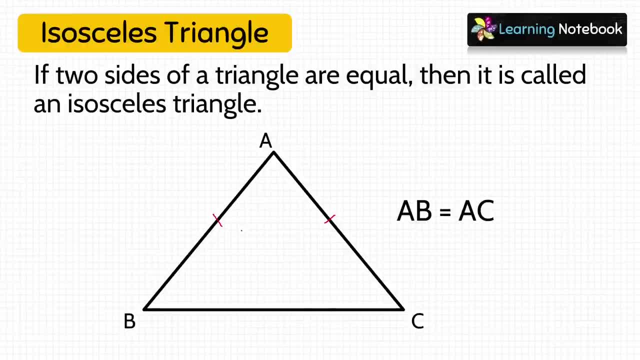 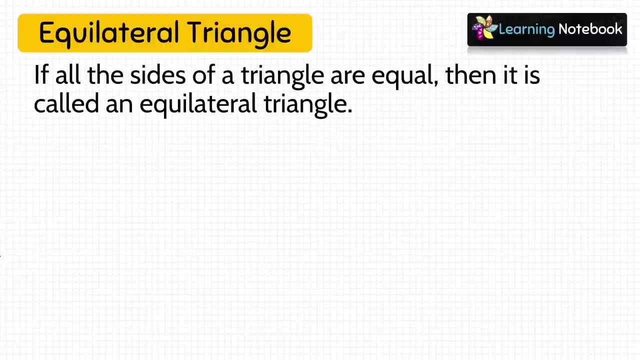 the isosceles triangle are always equal. So here angle opposite to AB is C and angle opposite to AC is B. So angle B equals to angle C. Second type of triangle is equilateral triangle. If all the sides of a triangle are. 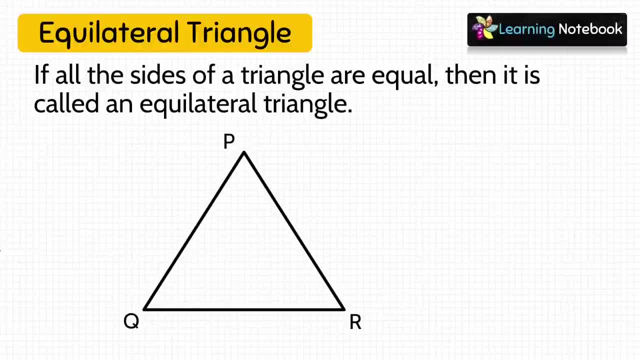 equal, then it is called an equilateral triangle, Like here in triangle PQR. PQ equals to QR equals to RP. It means all the sides of triangle PQR are equal. So this is an equilateral triangle Again. another important property to note here is: 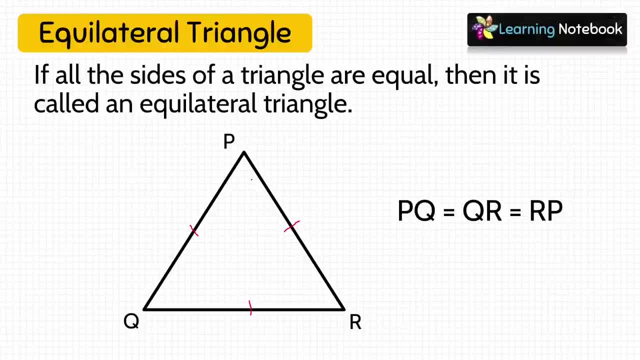 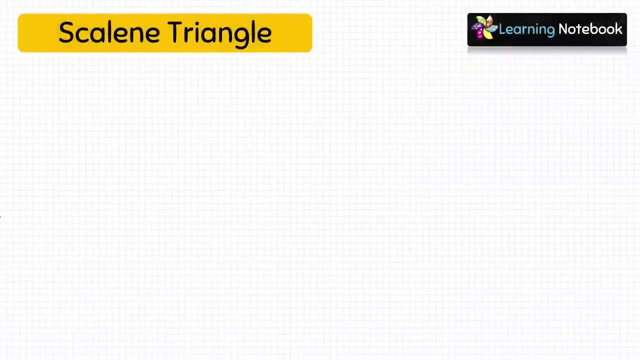 that all angles of an equilateral triangle are equal. So it means angle P equals to angle Q equals to angle R And since all the angles are equal, measure of each angle is 60 degree. The third type of triangle is scalene triangle. 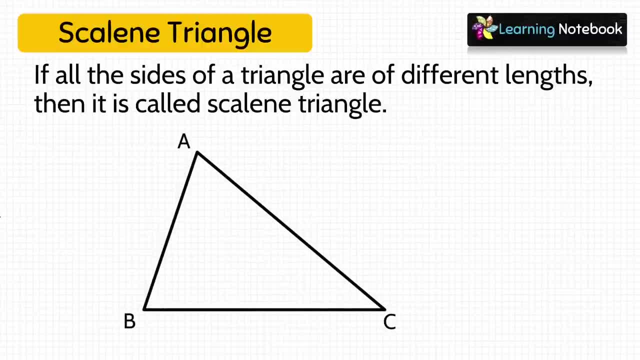 If all the sides of a triangle are of different lengths then it is called a scalene triangle, Like here: in the given triangle, ABC, AB is not equal to BC, which is not equal to AC. So it is a scalene triangle as all the sides are of different lengths. 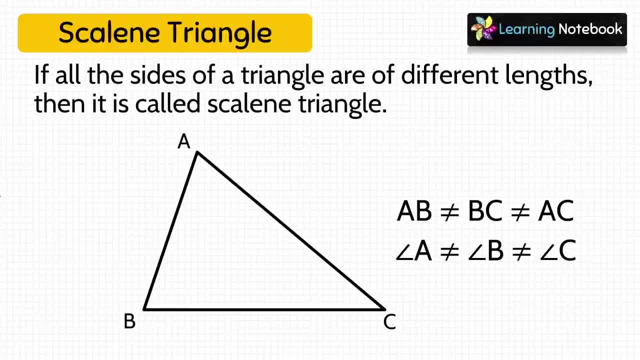 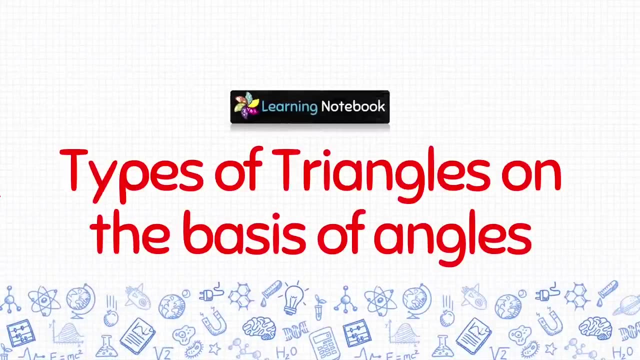 So all the angles of this scalene triangle will also be different. That is, angle A is not equal to angle B, which is not equal to angle C. So these were the three types of triangles on the basis of sides. Now let's learn about types. 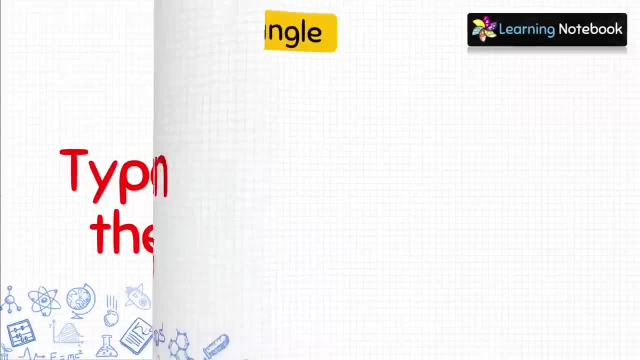 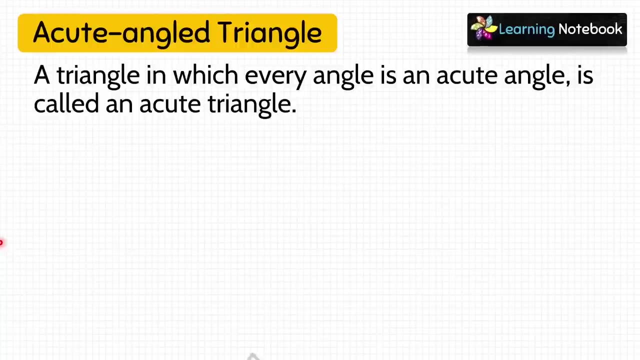 of triangles on the basis of angles. First type of triangle is acute angled triangle, Or simply we can call it as acute triangle, A triangle in which every angle is an acute angle. Such triangle is called an acute triangle. So here consider this triangle. 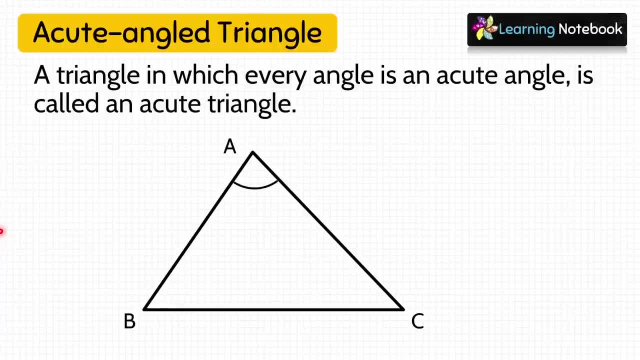 ABC, where angle A equals to 75 degree, angle B equals to 60 degree and angle C equals to 45 degree. So every angle of this triangle ABC is an acute angle, That is, each of them is less than 90 degree. Therefore, this triangle 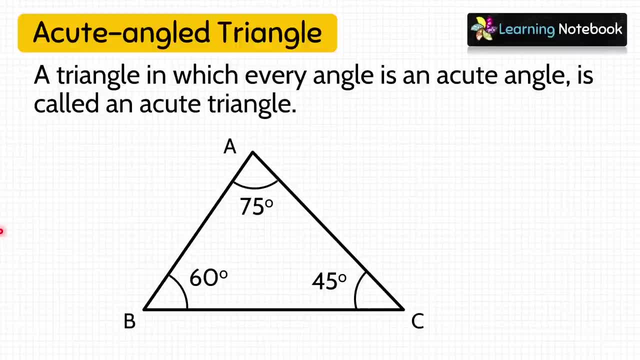 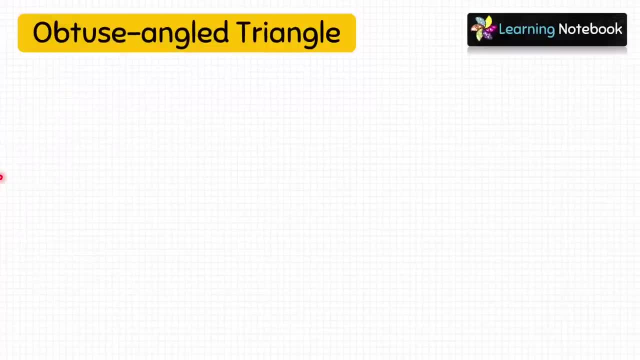 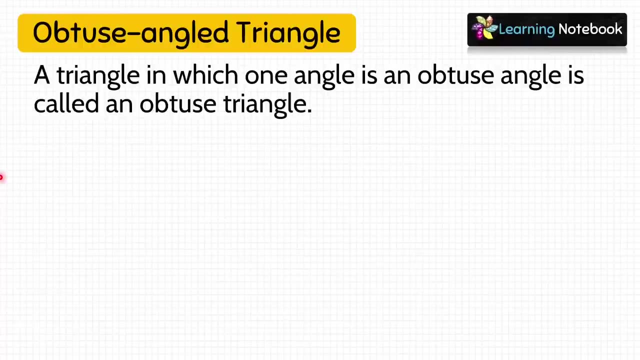 ABC is an acute triangle, or we can call it as acute angled triangle. Second type of triangle is obtuse angled triangle, or simply obtuse triangle, A triangle in which every angle is an obtuse angle. Such triangle is called an obtuse triangle. 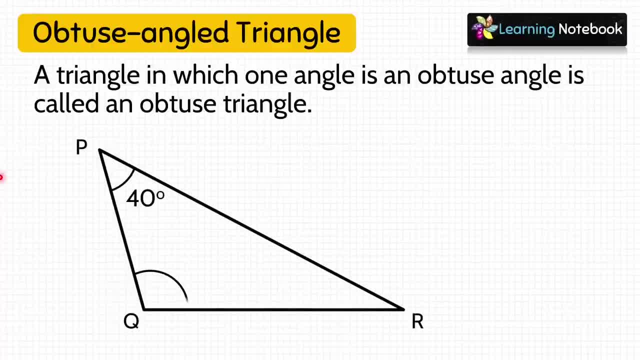 Like here in this triangle PQR, you can see that angle Q equals to 110 degree. So angle Q is an obtuse angle, as it measures more than 90 degree but less than 180 degree. So since one angle is an obtuse angle, so triangle. 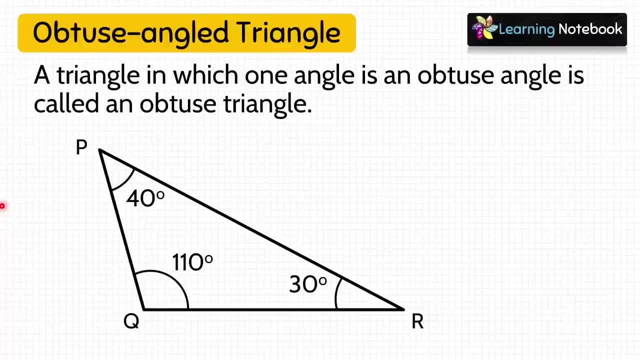 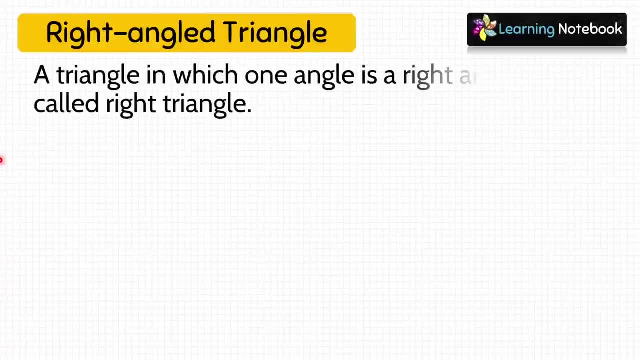 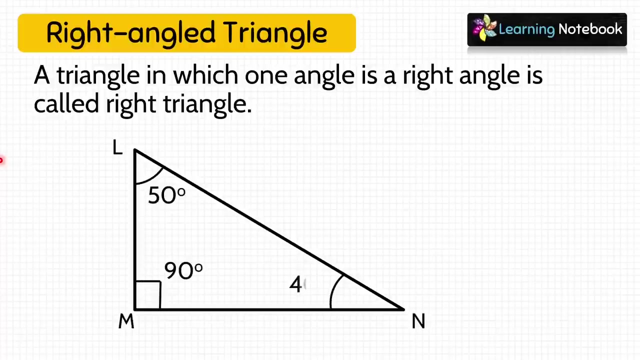 PQR is an obtuse triangle. And the last type of triangle is right angled triangle, A triangle in which one angle is a right angle. such triangle is called right angled triangle or simply right triangle. For this, consider this triangle LMN Here, angle M. 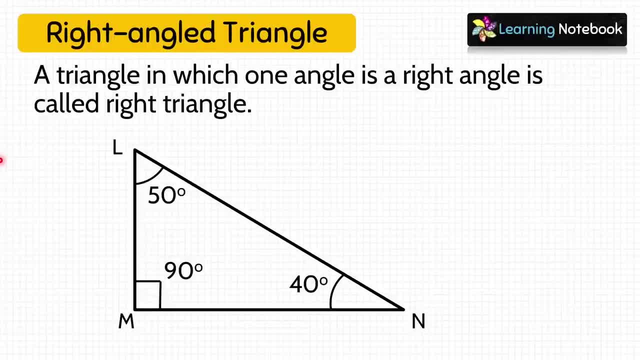 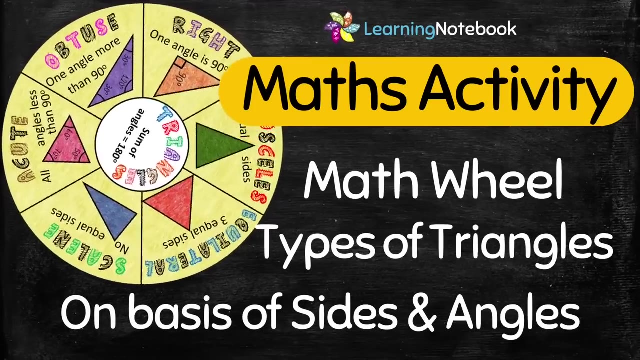 equals to 90 degree. That means angle M is a right angle. Therefore, triangle LMN is a right angled triangle. So, students, these were the three types of triangles on the basis of angles. Students, we also have a very interesting related activity on types of triangles. 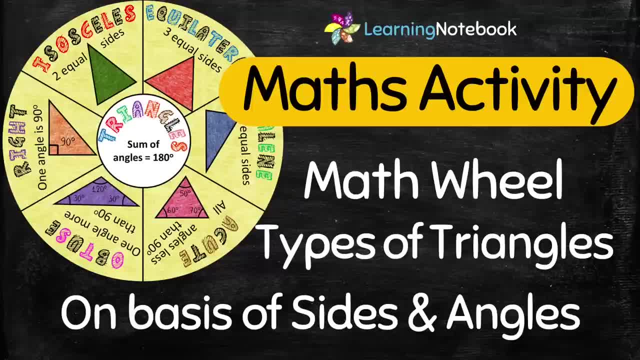 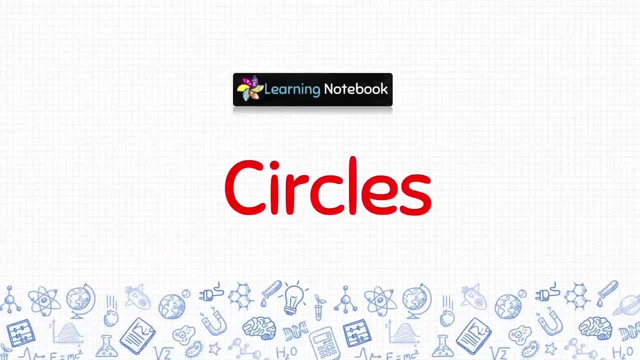 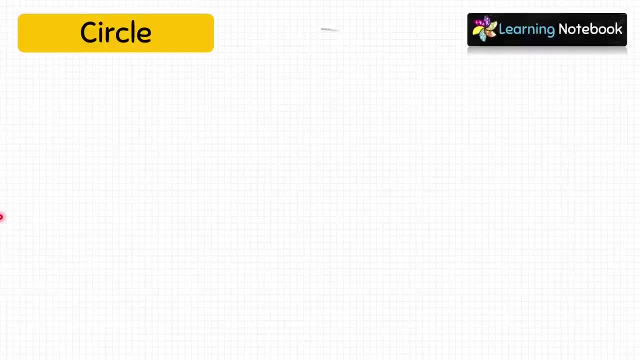 on the basis of sides and angles. I would suggest you to watch this video Now. our next topic is circles. So what is a circle? A circle is a simple, closed curve where all the points of the circle are at the same distance from its center. 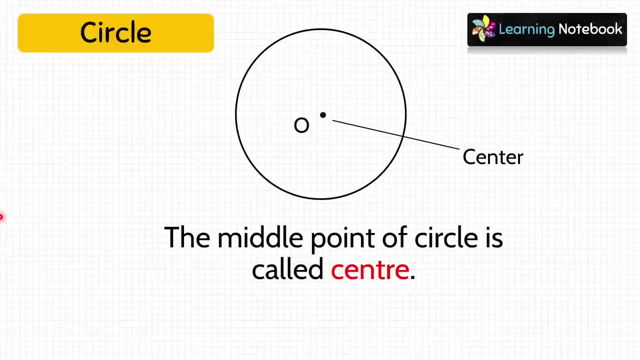 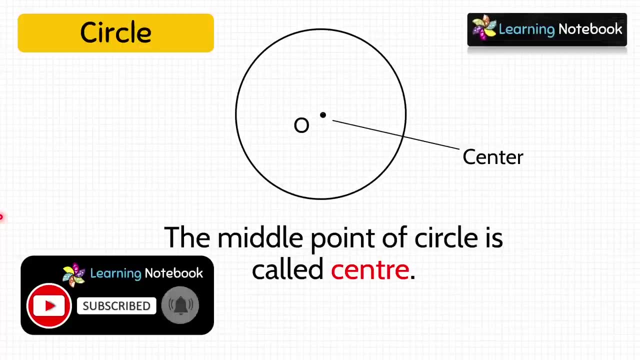 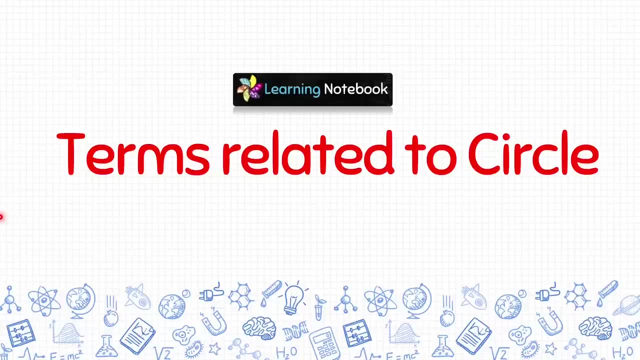 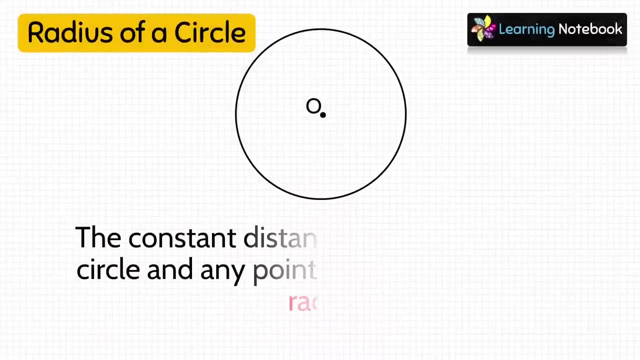 And the middle point of the circle is called the center of the circle. Like here, point O is the center of this circle. Now let's understand the terms which are related to circle: Radius of a circle. So what is radius of a circle? The constant distance. 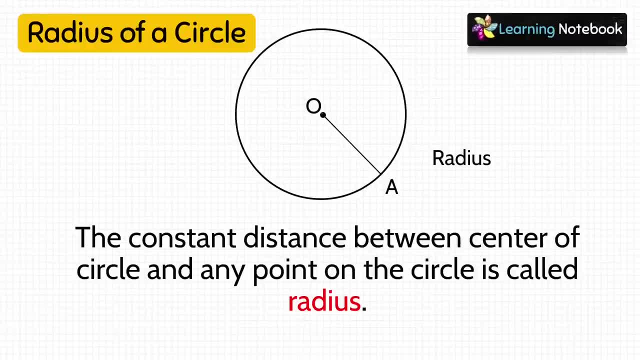 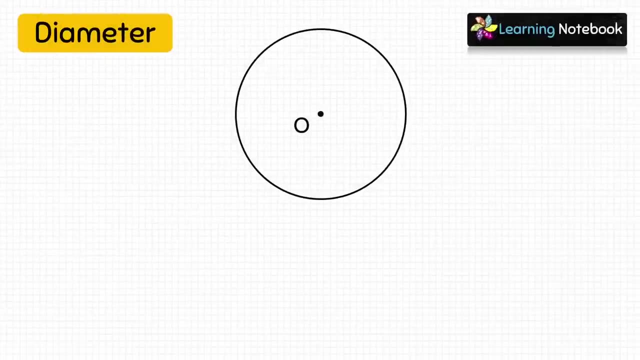 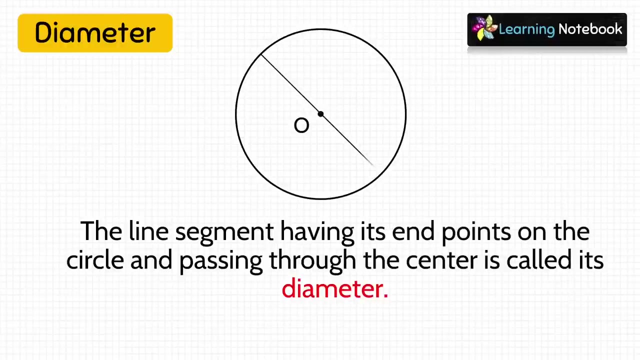 between center of circle and any point on the circle is called radius of the circle. So here OA is the radius of this circle. Another term which we learnt in class 4 is diameter: The line segment having its end points on the circle and passing. 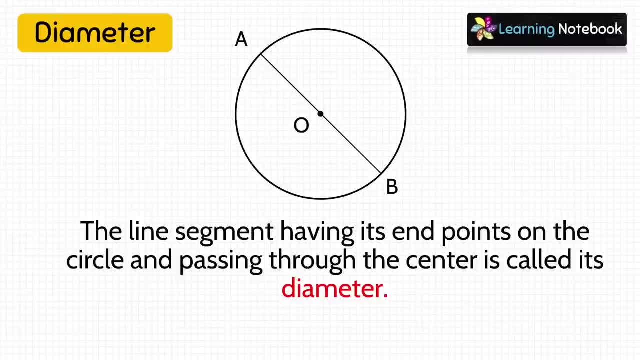 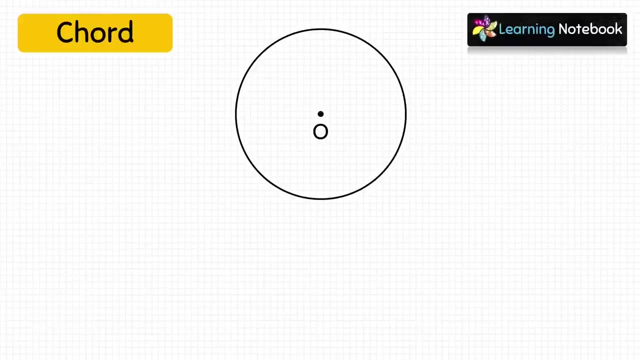 through the center is called its diameter, Like here in this circle. AB is the diameter of the circle And we also know that the relationship between diameter and radius is: the diameter equals to 2 into radius. Now next term is chord, which is new for you. So what is chord? 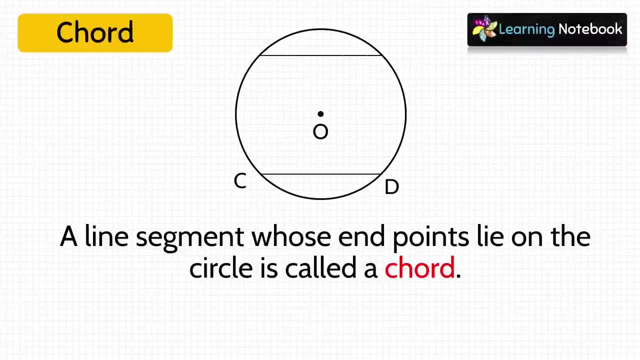 A line segment whose end points lie on the circle is called a chord, Like here, CD is a chord because both the points lie on the circle. Similarly, EF is also a chord, And I just told you that diameter also has both the points lying on the circle. 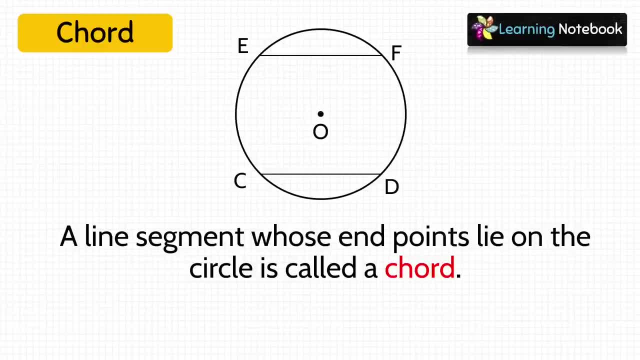 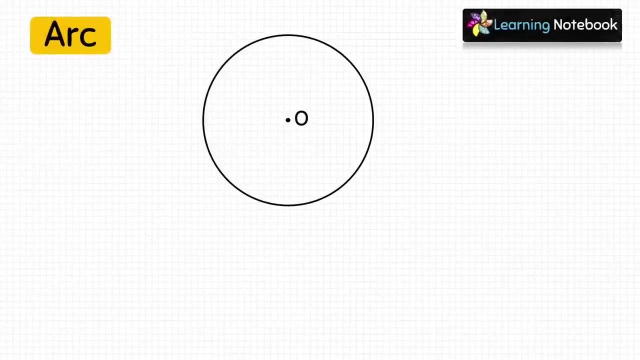 So is diameter a chord of the circle? Yes, the diameter is also the chord of the circle. In fact, the diameter is the longest chord in a circle. So here, EF, AB and CD, all are chords of the circle. Now another new term for you is: 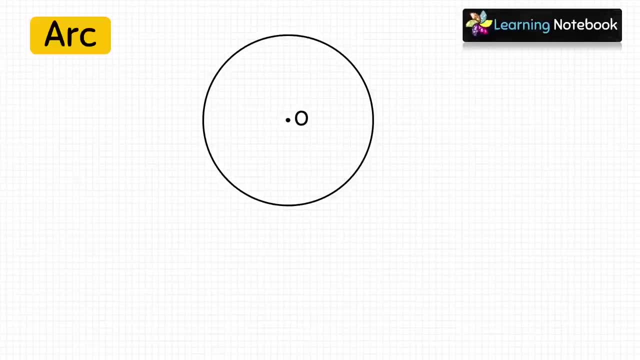 arc. Any part of a circle is called an arc of the circle. Like here, the highlighted part in red is the arc of this circle. Now, how to name this arc? We need three points to name an arc, So let's take P Q. 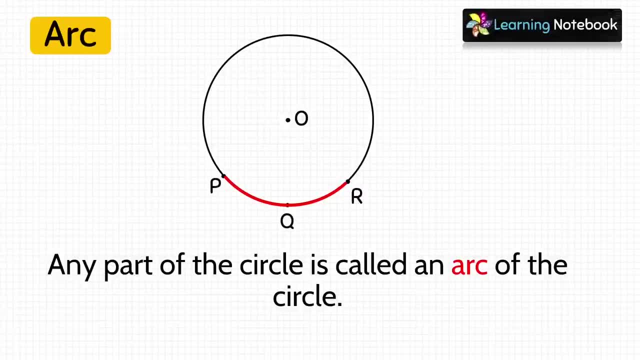 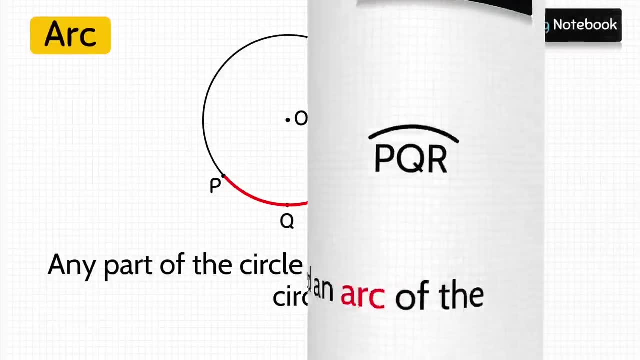 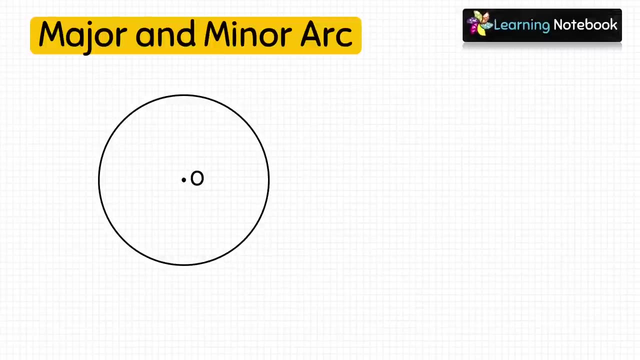 and R as the points. So we will write this as arc, PQ, arc. Now, next is major and minor arc. This is the circle here. Let's take any two points on this circle: P and R. These points divide the circle into two parts. 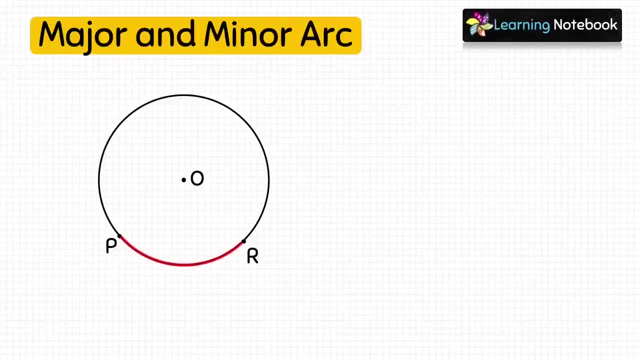 One is the shorter arc, which is called the minor arc, highlighted in red here, And the other part is the longer arc, which is called major arc, highlighted in green here. Now let's name both of them. To name the arc, we need three points. 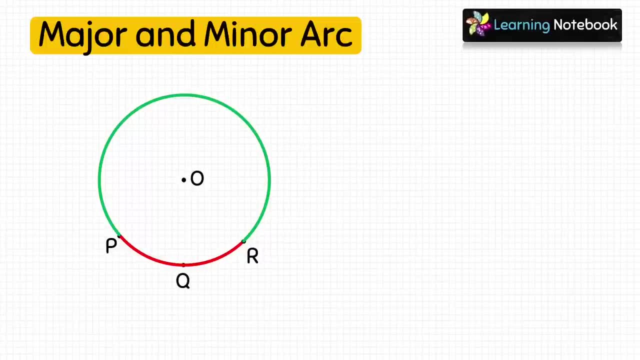 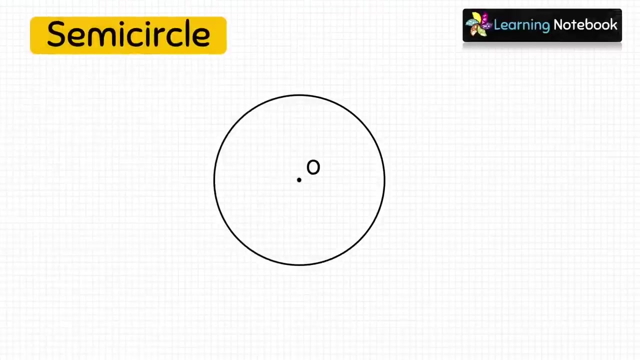 So first let's take point Q, So the minor arc is PQ arc. Similarly, let's take point T, on the longer arc, So major arc is PTR. Now next term is semi circle. Half of a circle is called a semi circle. 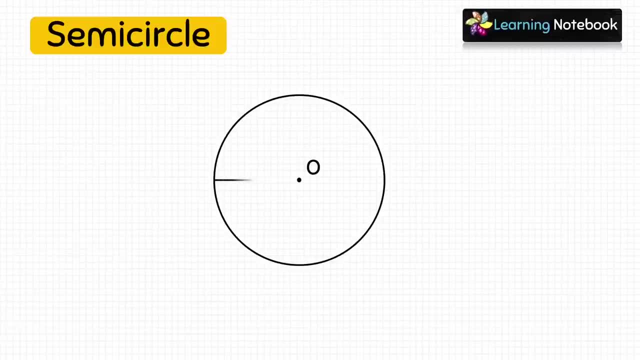 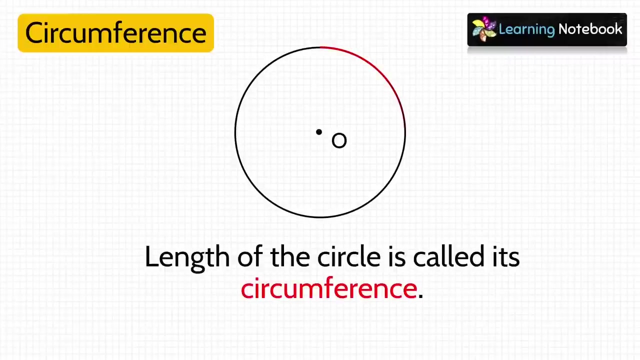 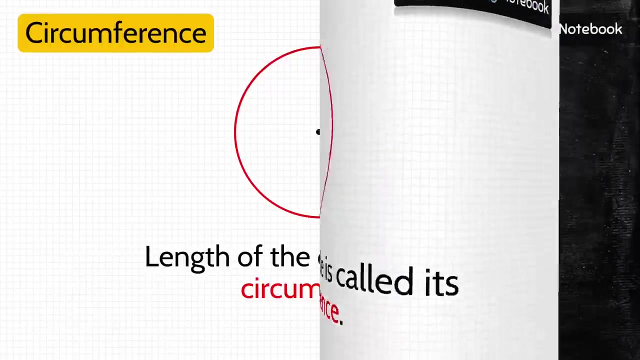 So to get a semi circle, let's draw any diameter AB. This diameter divides the circle into two equal parts and both the parts are called semi circles. Now, next term is circumference. Length of the circle is called its circumference. Now, students, let's do a. 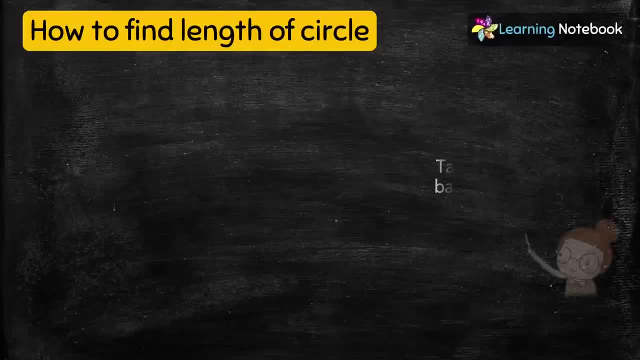 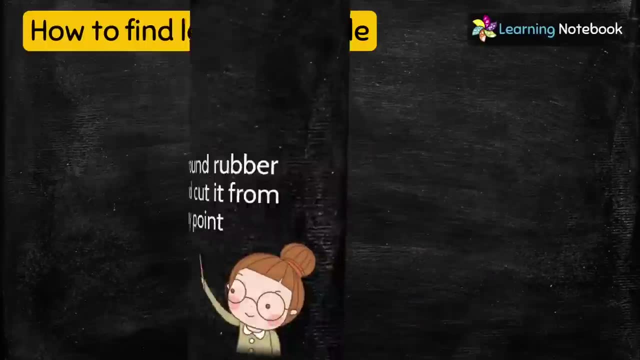 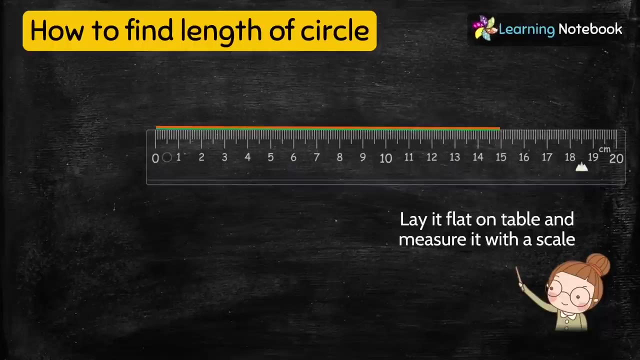 small activity on how to find length of a circle. For this, take a round rubber band and cut it from any point. Now lay it flat on the table and measure it with the help of a scale, As you can see the length of this rubber. 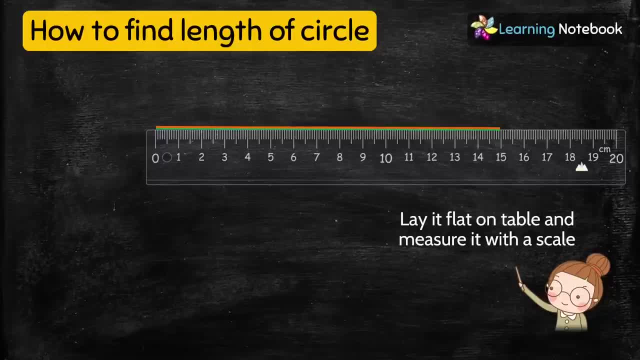 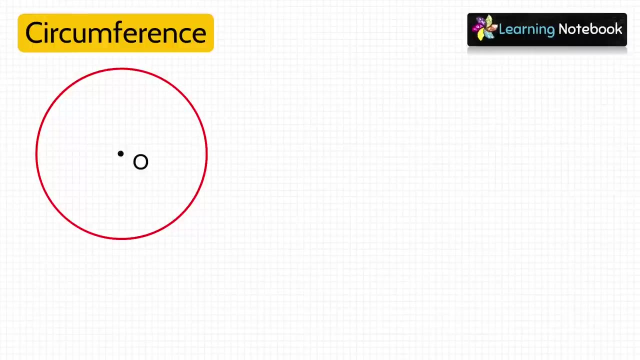 band is 15 cm. So this is the length of the circle, or its circumference. Now let's see how to measure circumference of a circle. To measure circumference of a circle we will use the formula that circumference equals to 2 pi r, where r is 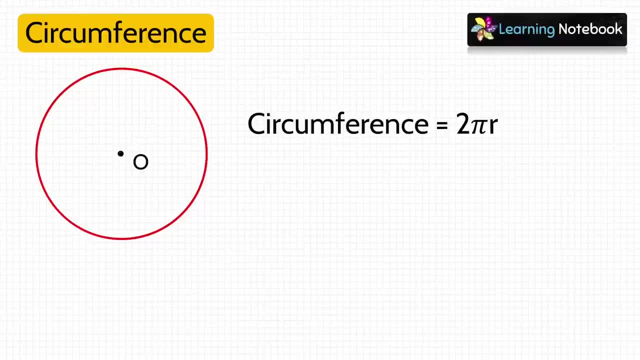 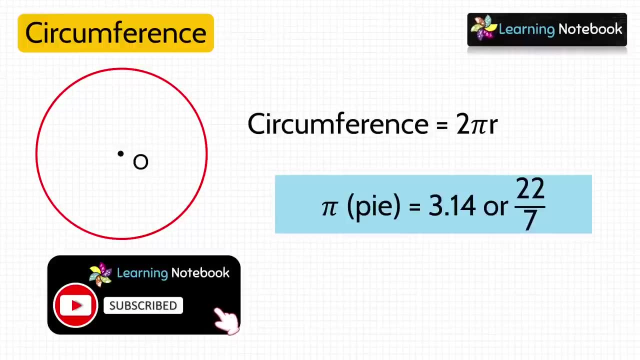 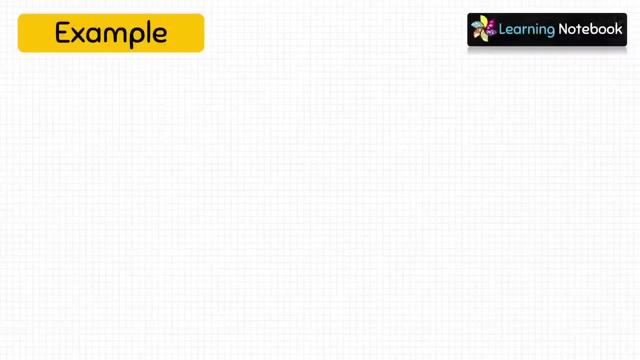 the radius of the circle and value of pi equals to 3.14 or 22 by 7.. Now let's solve some related questions. Question is: find the circumference of a circle whose radius is 3.5 cm and take the value of pi as. 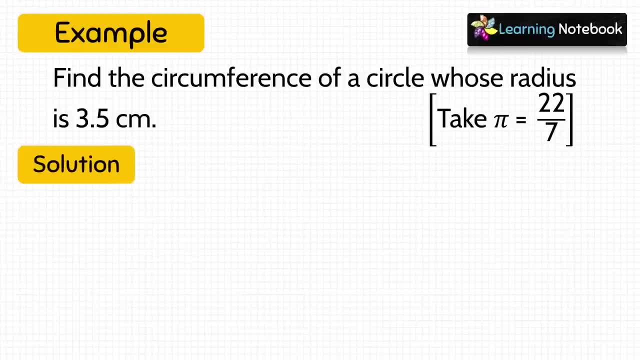 22 by 7.. So let's solve this question. We are given radius of the circle as 3.5 cm, Since the value of pi is given in fraction. so we have to convert this radius, which is given in decimals, into fraction. So let's 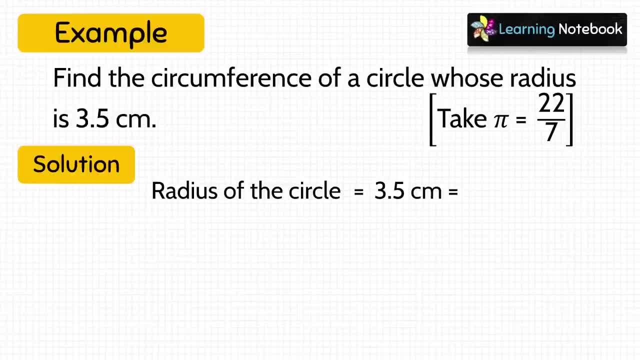 convert it: 3.5 equals to 35 by 10, which is equals to 7 by 2 cm. Now we just learnt that circumference of a circle equals to 2 pi r, So let's put the value of pi as well as. 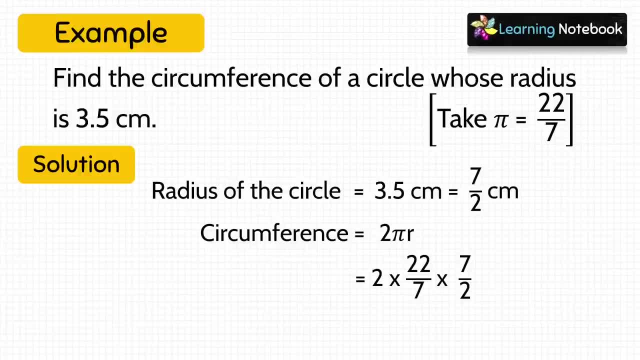 r here We get 2 into 22 by 7, into 7 by 2.. Simplify it: Cancel 7 by 7 and 2 by 2. We get 22.. So circumference of this circle is 22 cm. 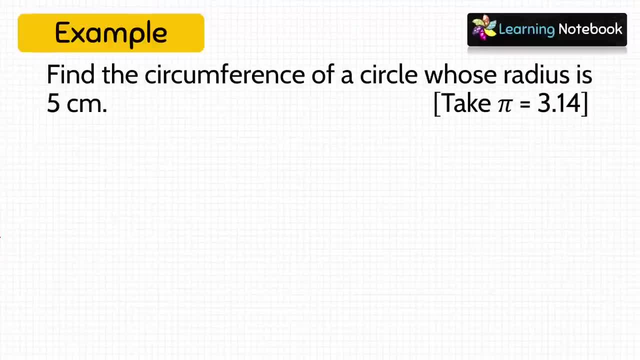 Let's solve one more question. Find the circumference of a circle whose radius is 5 cm And take the value of pi as 3.14.. So let's solve this question. We are given that radius of circle is 5 cm. 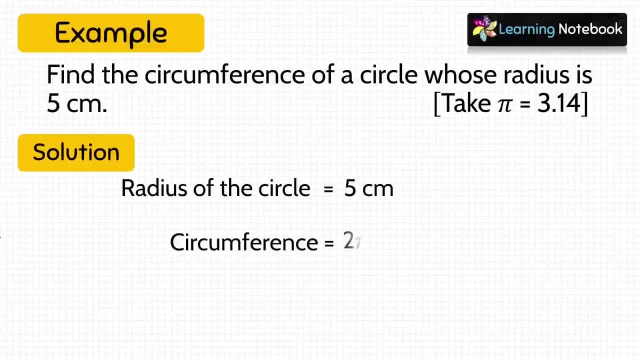 And we know circumference of a circle equals to 2 pi r. So let's put the value of pi and radius here, We get 2 into 3.14 into 5.. Multiply the numbers and we get the circumference as 31.4 cm. 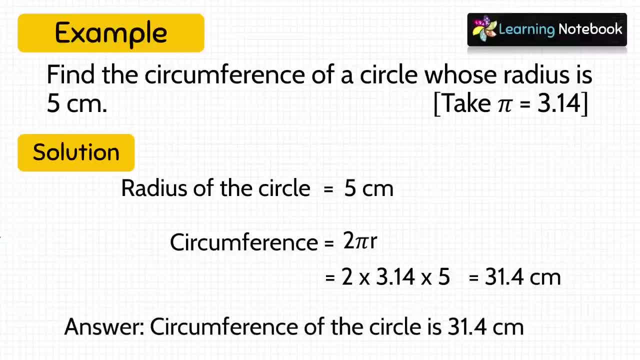 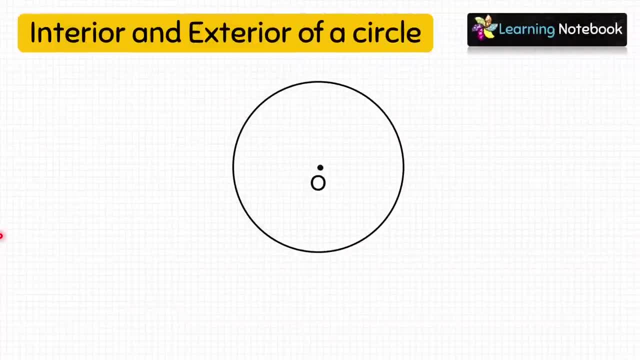 So answer statement will be: circumference of the circle is 31.4 cm. Now let's understand what is interior and exterior of a circle. Consider a circle with center O and take few points: P, A and M. Now, students, point P is inside the circle, So 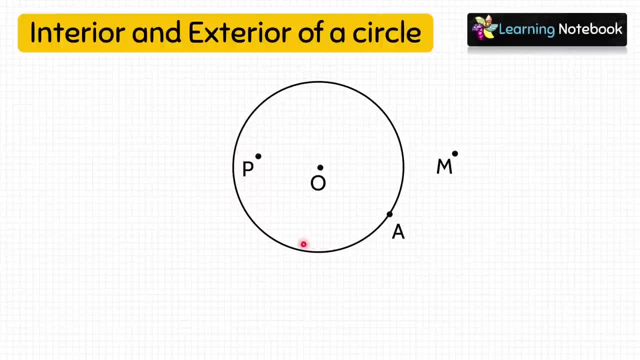 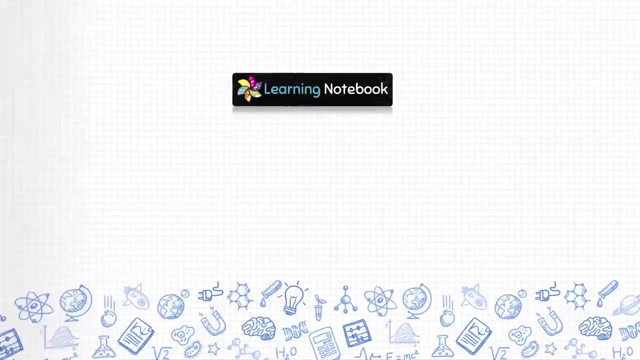 it lies in the interior of the circle. Now look at point M. It lies outside the circle. So we will say point M lies in the exterior of the circle And point A it lies on the circle. Now let's understand how to draw a circle with the 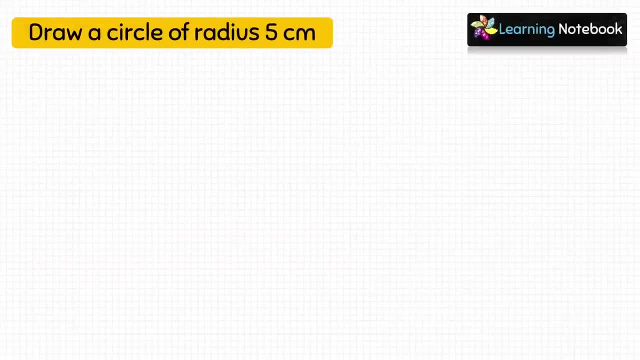 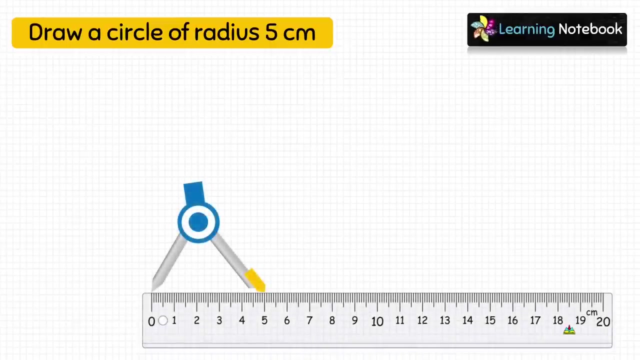 help of compass. Let's draw a circle of radius 5 cm For this. take the compass and keep its needle at 0 of the scale. Now open the compass to measure the required radius, which is 5 cm in this case. Now students. 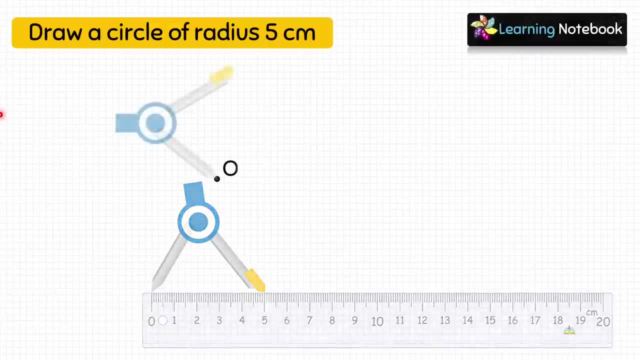 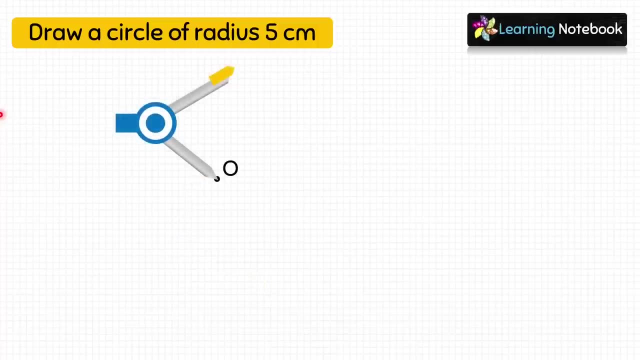 mark a point O on the plane of the paper and rest the metal tip of the compass firmly at O. Next hold the head of the compass firmly and move the pencil point around to trace a circle of radius 5 cm. So here we have drawn a. 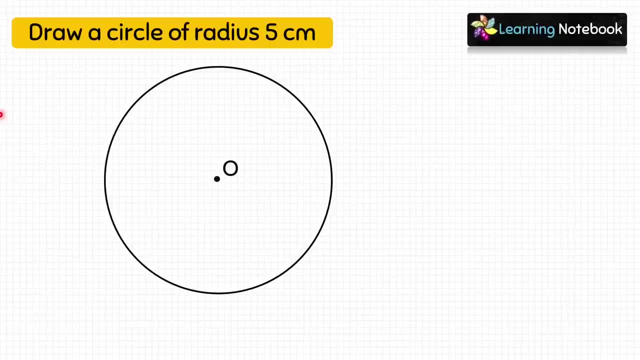 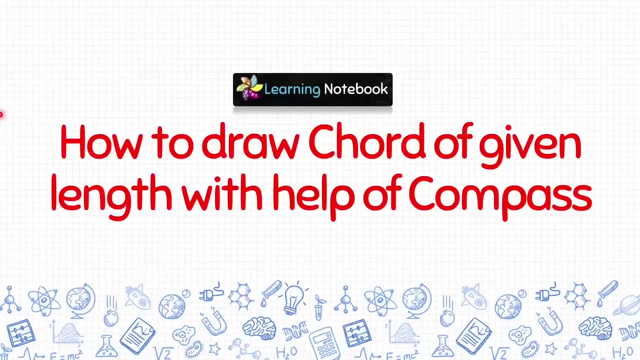 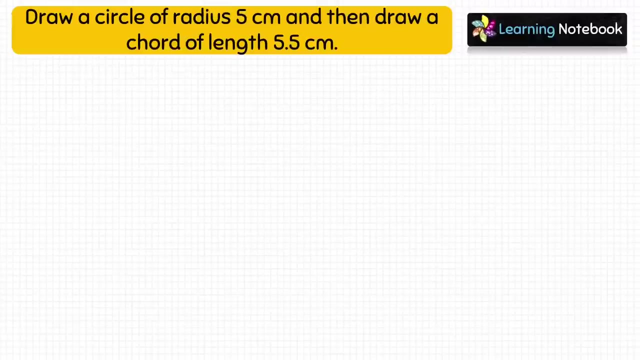 circle of radius 5 cm with the help of compass. Now let's see how to draw chord of given length using compass. So question is: draw a circle of radius 5 cm and then draw a chord of length 5.5 cm. So 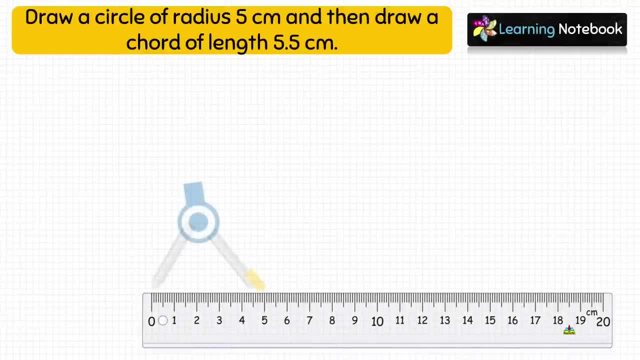 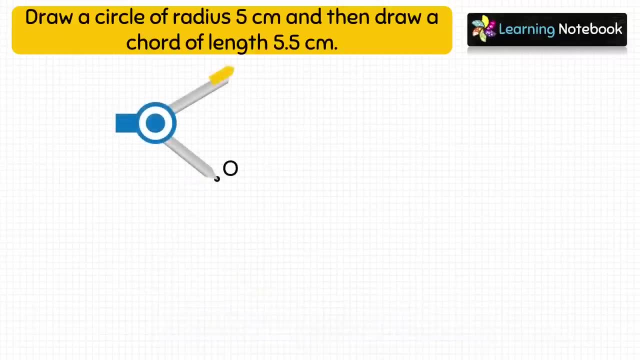 first we have to draw a circle of radius 5 cm. So let's follow the same steps as we did earlier and draw a circle of radius 5 cm. Now, students, to draw a chord of length 5.5 cm. open the compass to.